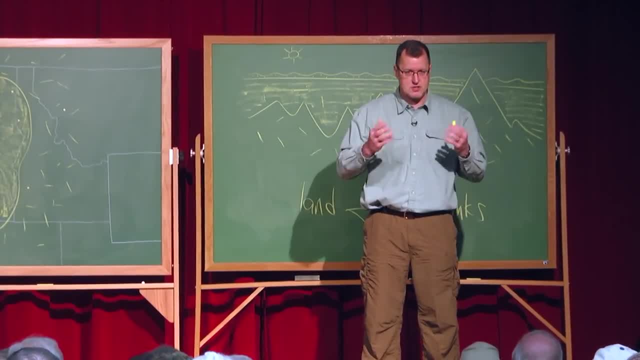 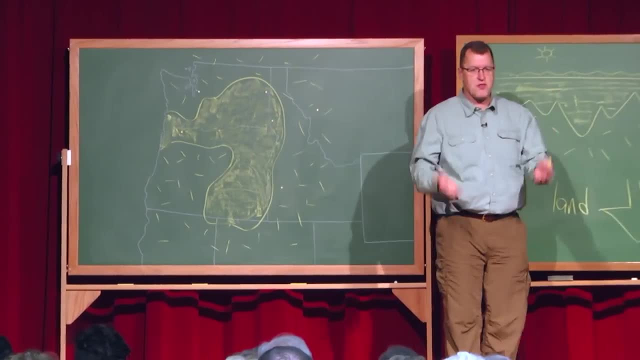 lavas or daysite lavas. These are different kinds of chemistries And these are basalts. Look at this map. Look at how much of the Pacific Northwest has this thick pile of basalt lava. It's nothing to do with the Cascades. Let's get that out of our minds right now. 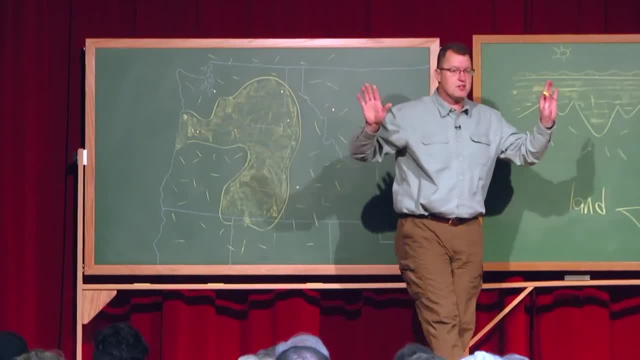 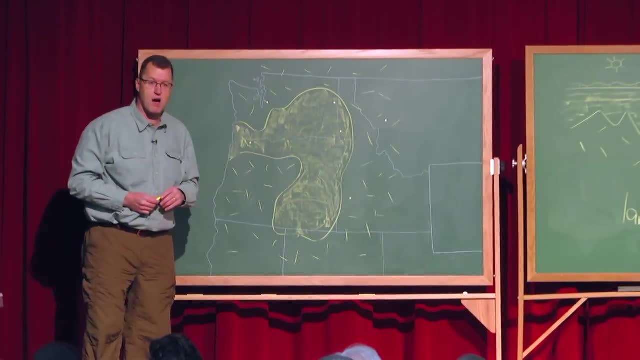 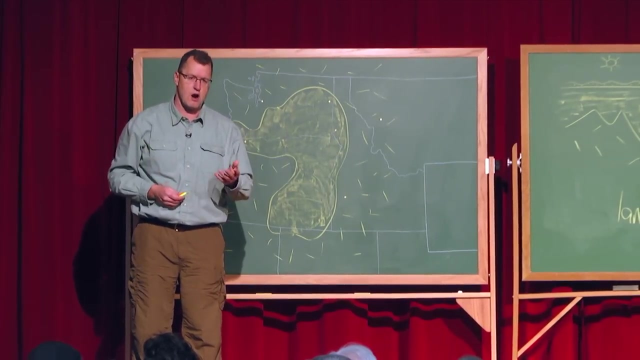 Mount Rainier, Mount Hood, I don't care. Nothing to do with tonight's talk. Is it true that these giant lava flows- and they are giant, Some of them traveled 300 miles, Some of them are more than 100 feet thick. Is it true that those lava flows are unusual? Sure, I mean. 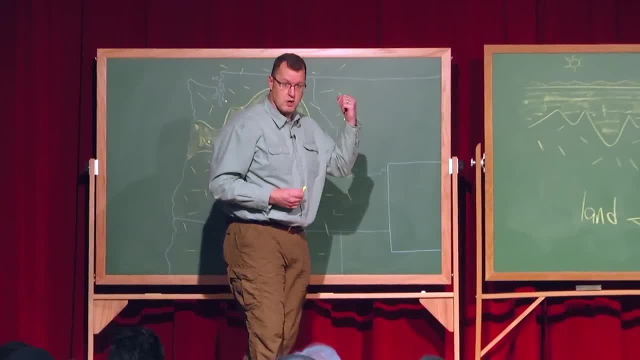 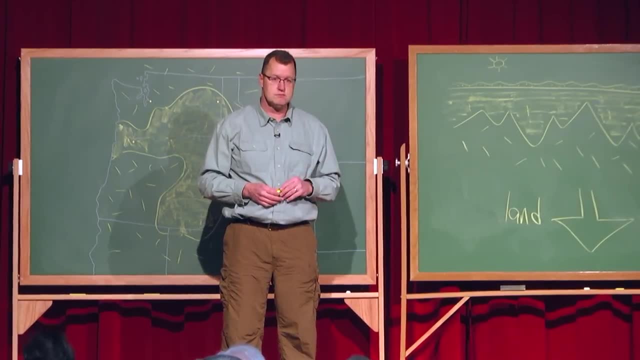 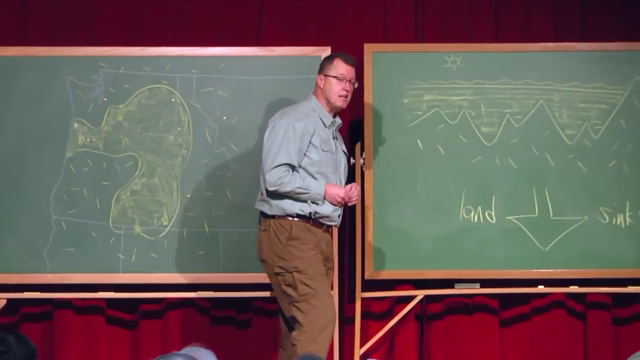 they're bigger than the lava flows you see in Hawaii or Iceland- where we're going to go tonight, by the way- But is this the only place in the world that we have these kinds of lavas? No, No. There are flood lavas like these in Siberia. There are flood lavas like these in India. 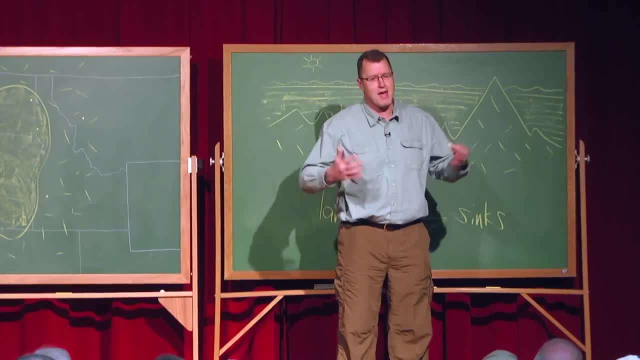 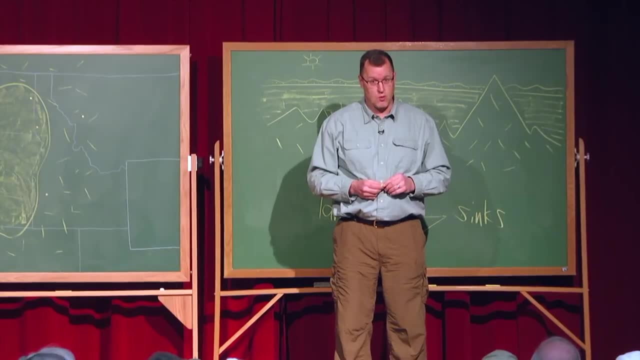 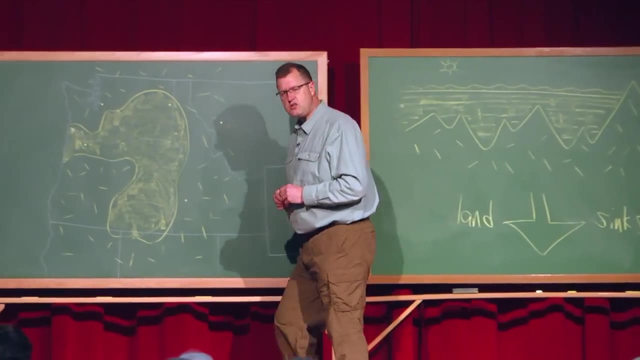 Well, okay, fine, But ours must be the biggest and the best, right, I mean, you know? No, We are small potatoes compared to these other flood basalt areas, And we will look at the volumes tonight as well. Have you heard this one? There's mass extinctions in our planet's history, where large percentages 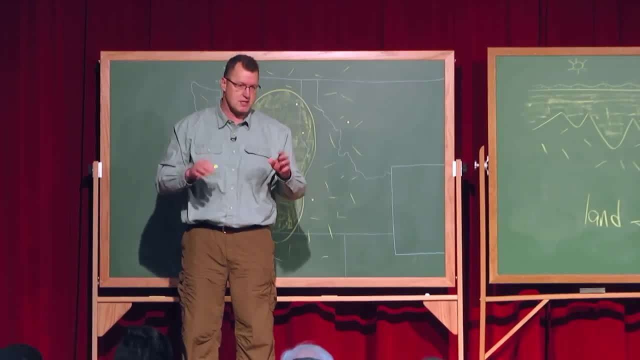 of all living things are destroyed And we're not going to be able to do that. We're not going to be able to do that. We're not going to be able to do that, We're not going to things disappear from the fossil record, Mass extinctions- You've heard of those, maybe. 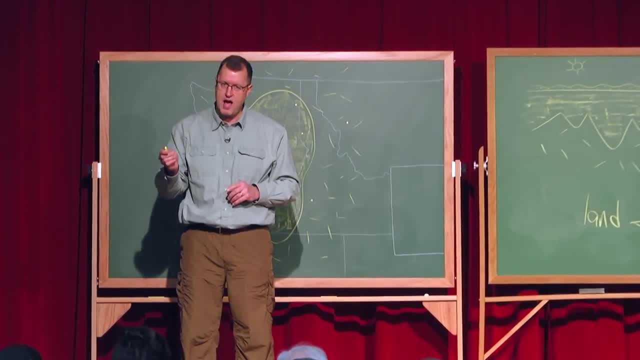 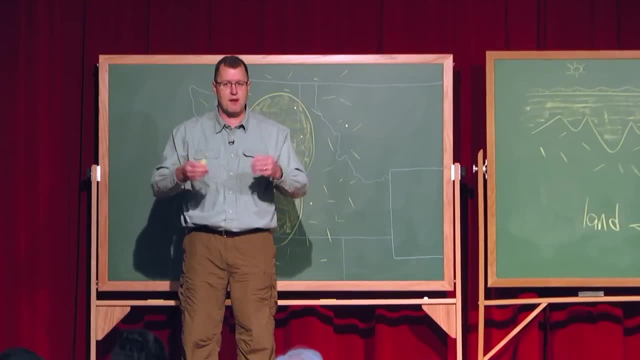 Have you ever heard that there's a connection between these flood lavas, the age of these flood lavas and these mass extinctions? Oh, some of you have Well good. Well, I'll expand on that as well. So we've got a lot to talk about in addition to the basic stuff I've 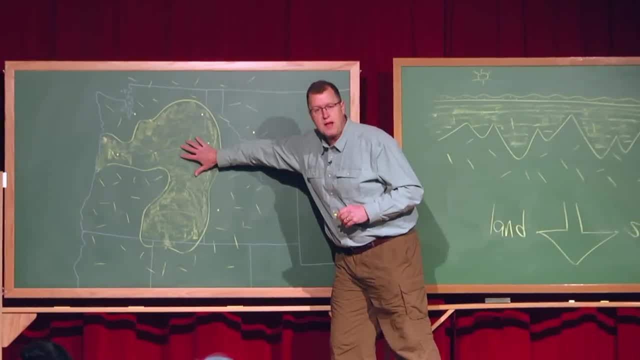 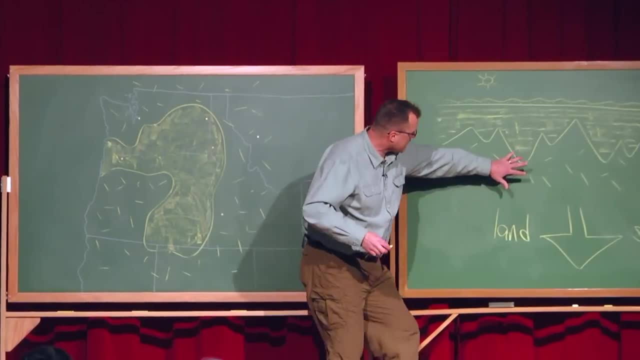 always done. One more introductory comment: This is just a big pile of lava surrounded by stuff that's not lava, essentially, And in this cross-sectional area we've got a lot of lava, And in this cross-section we can see this stuff here that's just buried beneath all. 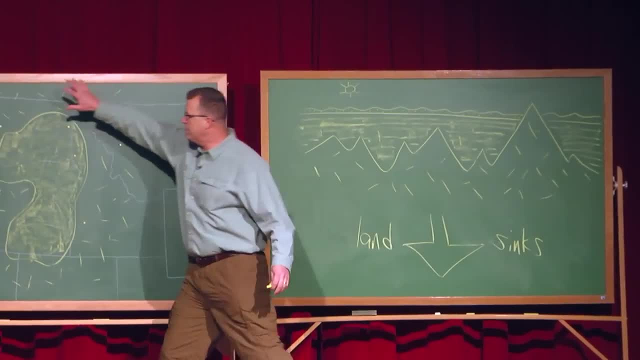 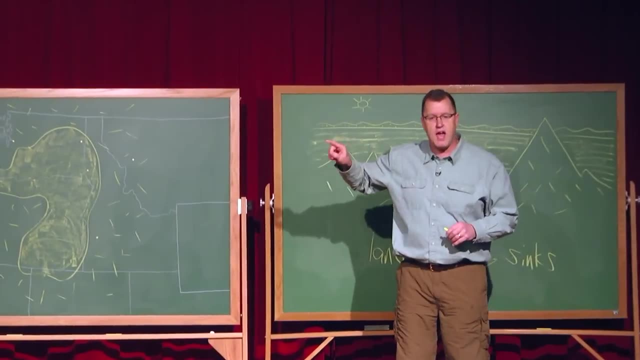 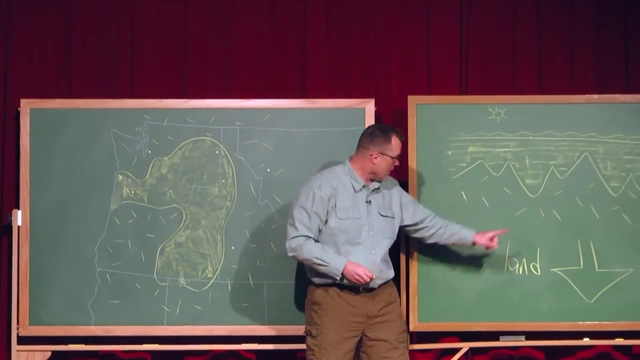 this lava. So if you are a geologist who loves all this old rock, all these metamorphic and granite rocks- and they tell all these old stories of Washington- you hate the Columbia River basalt lavas. If you are a person who loves all these rocks or loves all these, 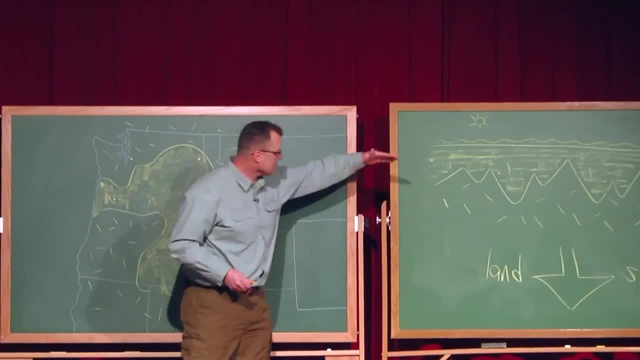 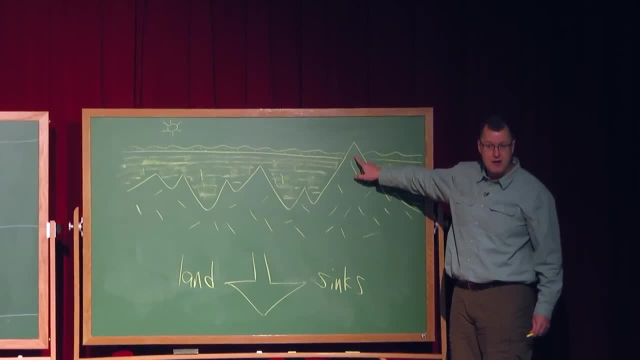 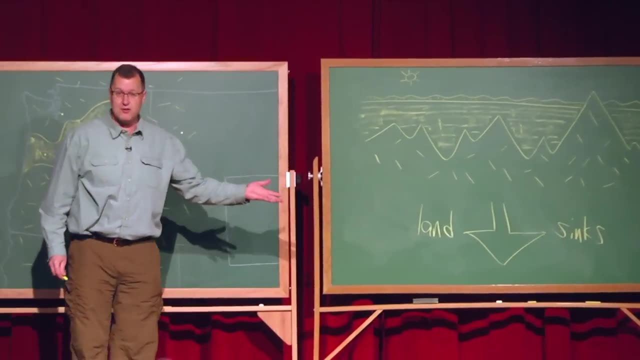 Columbia River States And all of theseBoth of the, because those have not buried everything That's called Steptoe Butte, over by Pullman. that's a mountain peak that kept its chin up above all of these lavas, But most of those mountains are still down there. 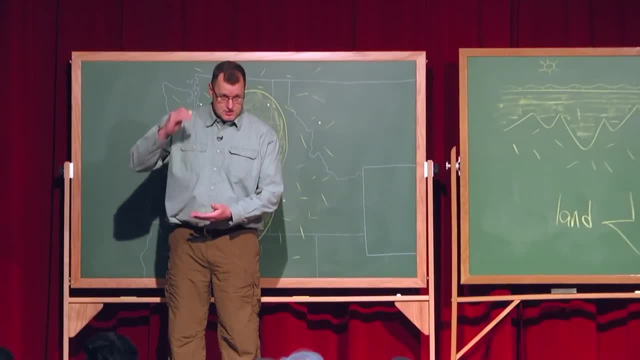 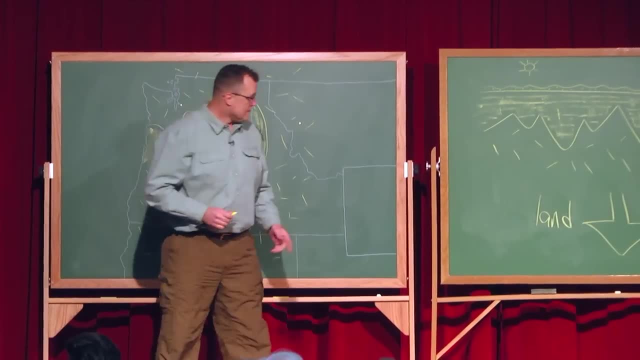 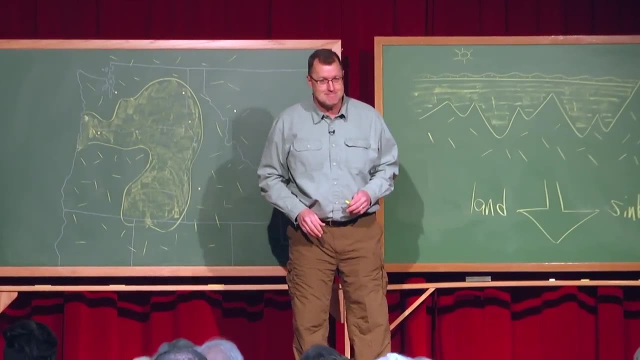 they're just under- and I'm not making this up now- two miles of lava, In some places more than three miles of lava. So I've heard on field trips geologists who love these other rocks talk to this as a big, giant cow pie. 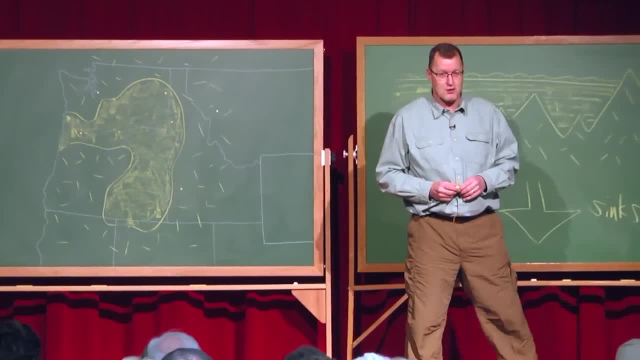 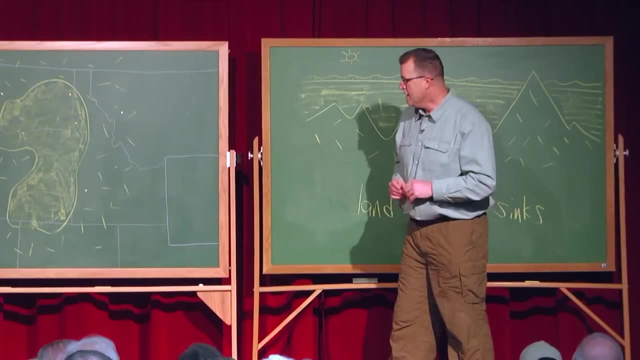 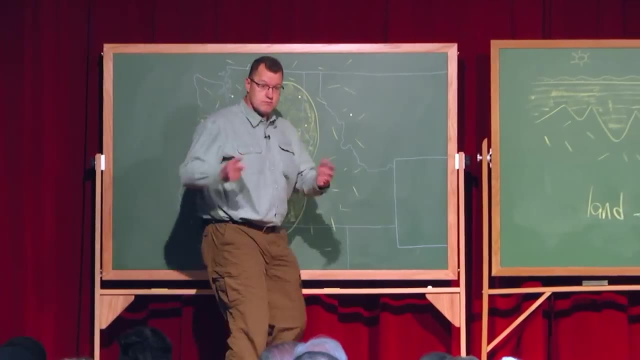 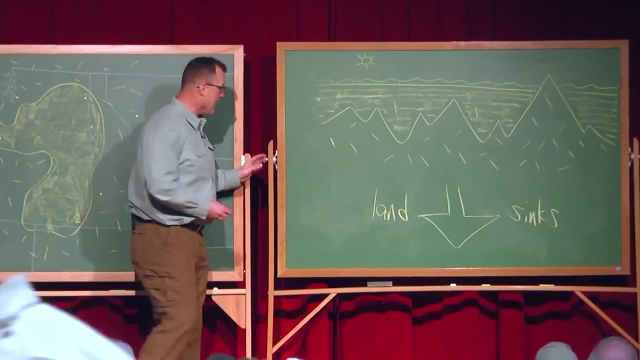 They're not a fan of our flood lavas, our great lavas of tonight. But some of you came into town. you had a beautiful meal downtown, so you don't want to talk about cow pies, and I understand. So let's not call it a cow pie, let's call it a German chocolate cake. How about that? Brown brown, rock brown. So this is the cake, These are the lavas. Somebody get that. 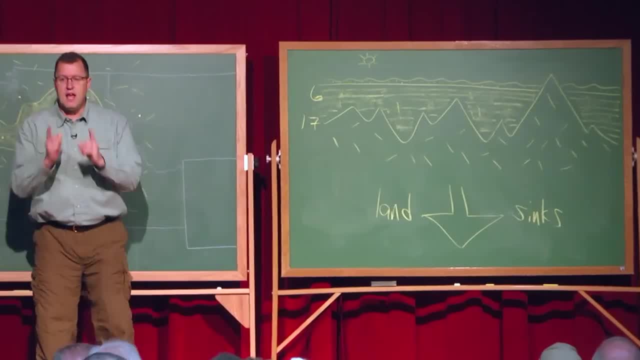 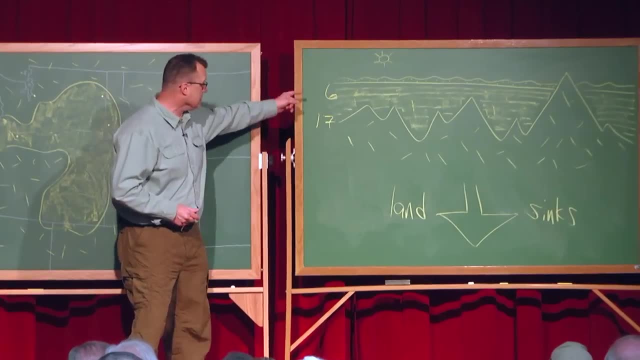 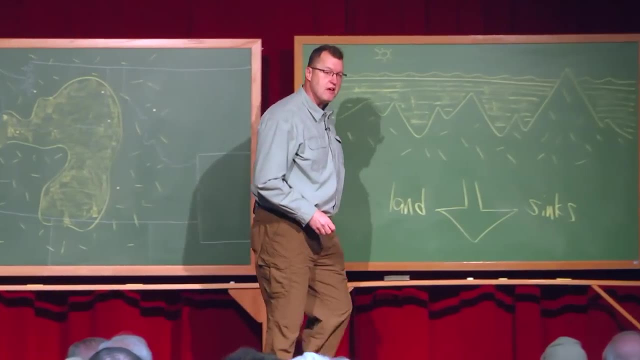 And the age of these eruptions is very specific. Seventeen million years ago is when these lavas began erupting. Six million years ago is when these lavas ended. Seventeen to six. We got a pretty good answer about what happened seventeen million years ago to start this eruption story. 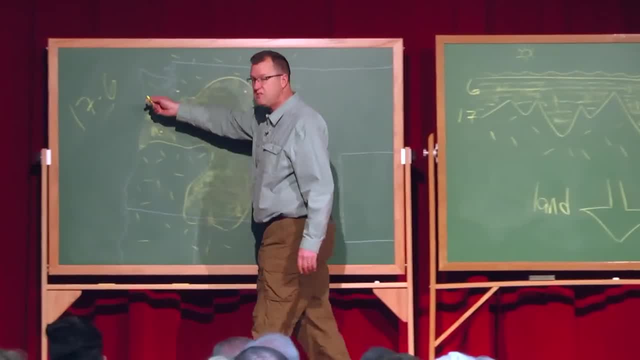 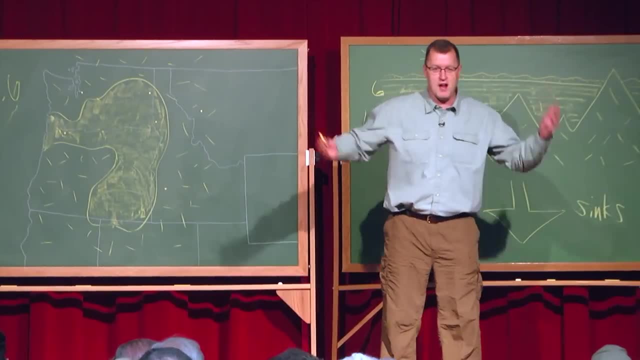 We have less of a satisfying answer to explain why the system stopped. But at least these eruptions aren't something you don't have to worry about. You know, most of these geology lectures don't have an answer. These lectures are some sort of terror thing. you know It's an earthquake and the thing's going to come in a landslide. 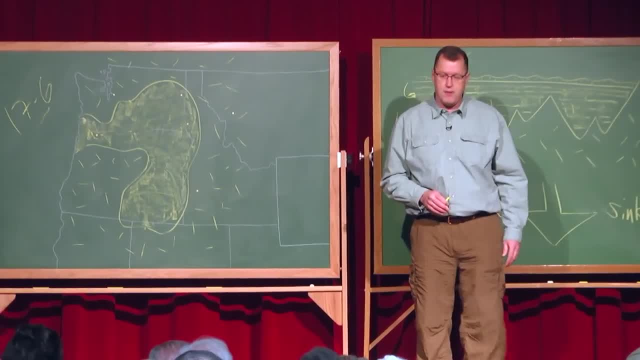 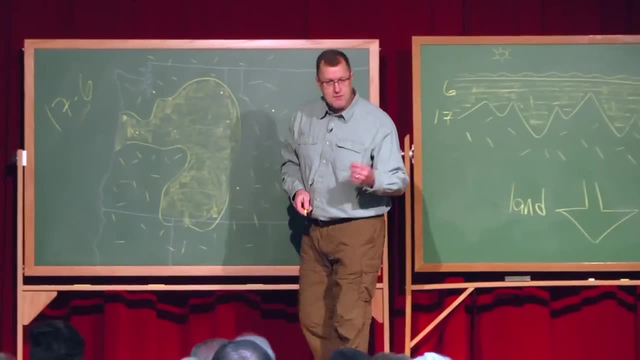 So this is all stuff tonight, just safely tucked in the past, and there's no chance in the foreseeable future we'll have any of these eruptions. A couple final comments from these images before we erase them and move on to something else. As I mentioned, these are mostly metamorphic and granite rocks. 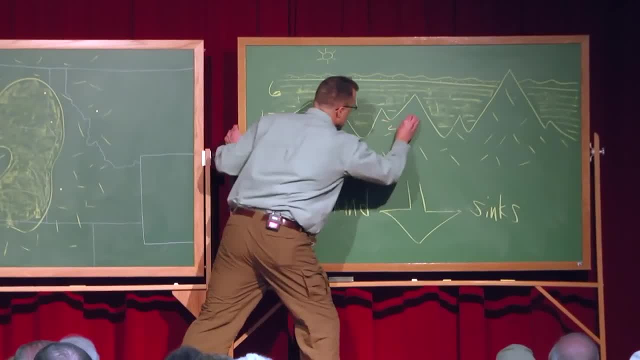 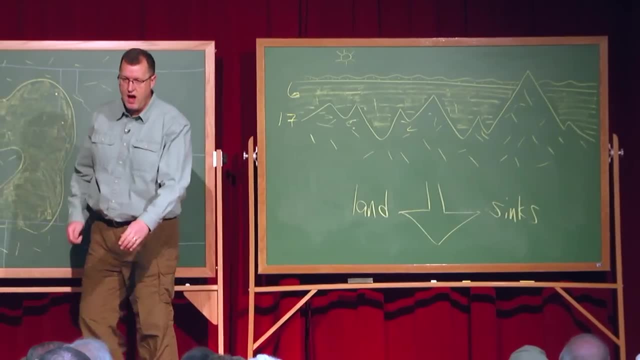 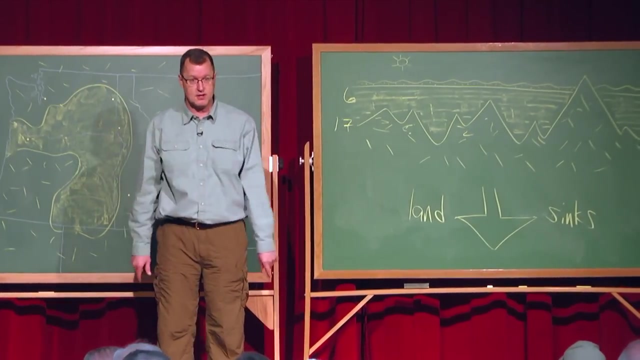 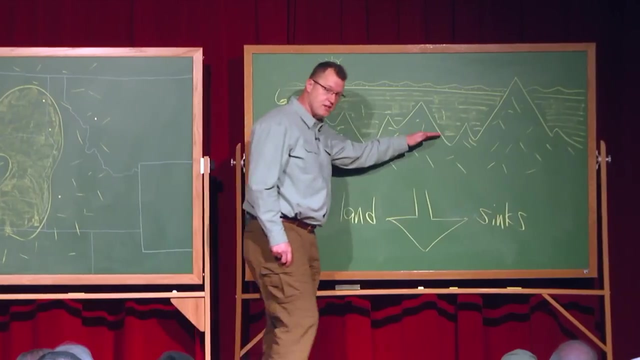 However, there's also, at the upper part of these old rocks, thick sections of sedimentary rock, The Swak Formation. Some of you know about the Swak Formation. We've talked about that in association with the Liberty Goldfields. So there are thick sections, thousands of vertical feet of sedimentary rock beneath many of these places, where our German chocolate cake is. 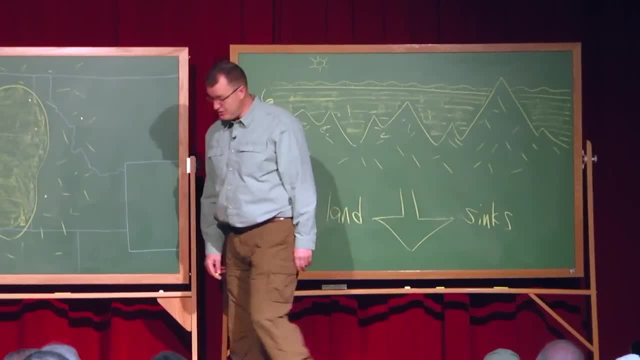 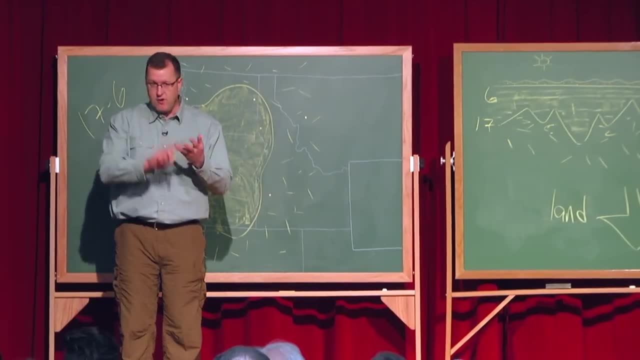 And the oil people have been here. They've been drilling, They've been looking for oil and natural gas. They were here in the 2000s, They were here back in the 1980s- Shell Folks from Canada. 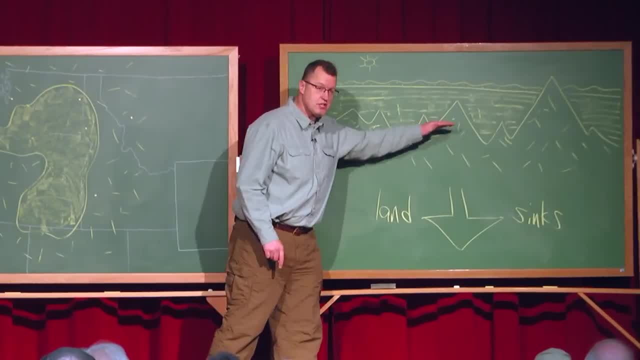 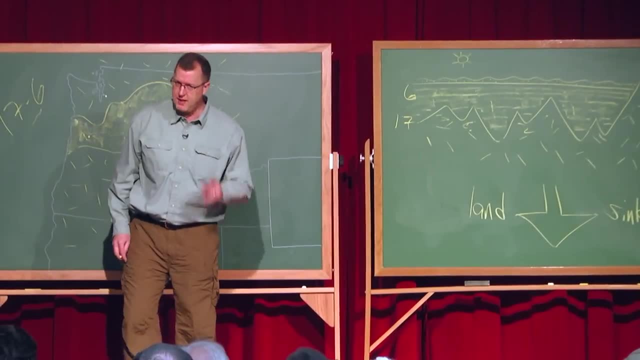 And they're probably coming back, Because there's enough indications that beneath this German chocolate cake there are large pools, large reservoirs of oil and natural gas- Depends on who you talk to- But that drilling has helped us understand exactly how thick these lavas are. 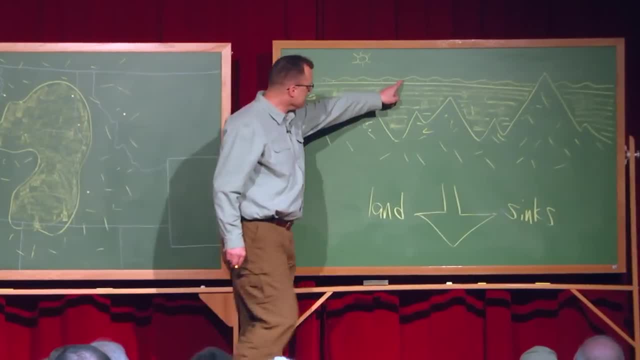 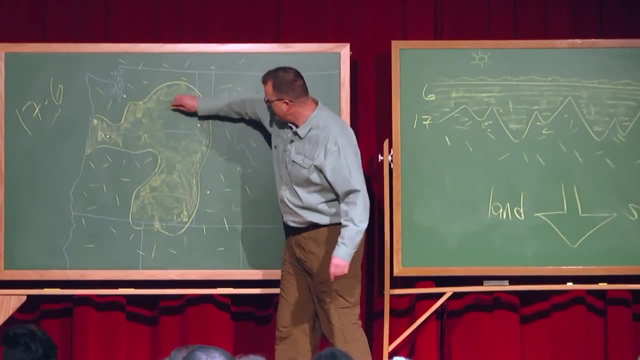 The top of the German chocolate cake. in places there's a bunch of dots here. This is Loess. This is wind-blown silt. It's kind of right here on this map: Loess is wind-blown silt. 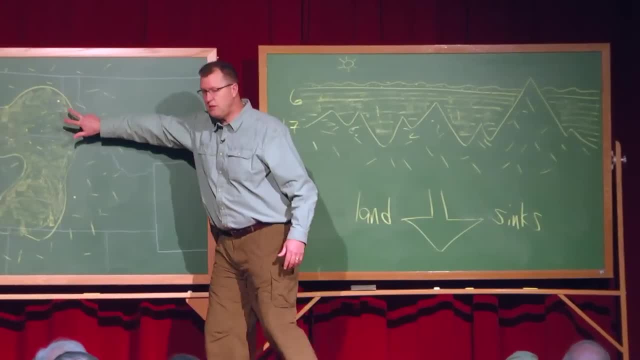 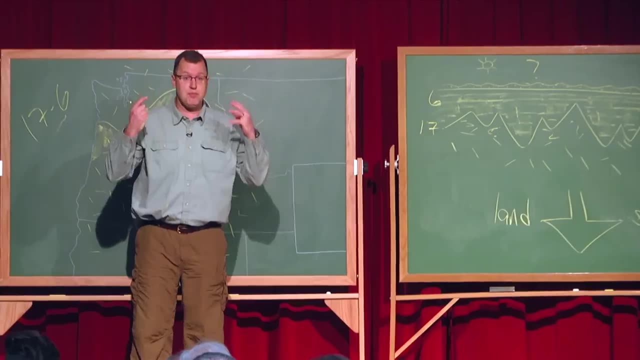 It's silt that blew in off the winds and got deposited. This is still a bit of a question mark even today. Where, ultimately, is the origin of the Palouse Hills? So that's what I'm talking about. So if you get towards Pullman, you know those rolling wheat fields and all that. 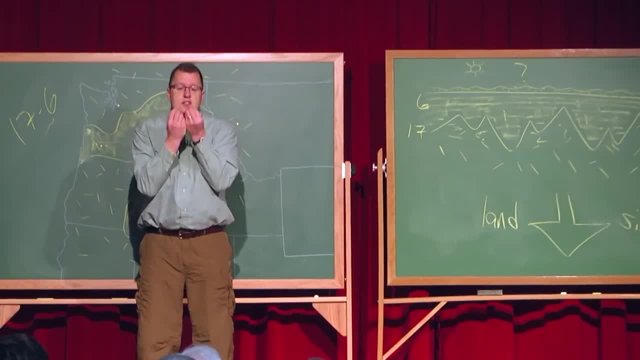 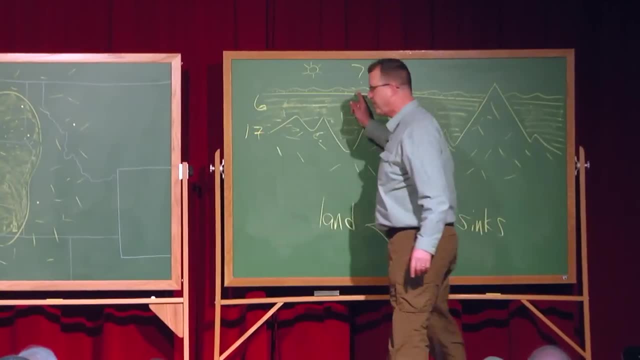 That's a unique landscape. Those hills are made out of this kitchen flour. Ultimately, it's still difficult to prove where that stuff came from. Yes, the Ice Age floods came and eroded some and redeposited, But I'm talking about, ultimately, where did that Loess come from to begin with? 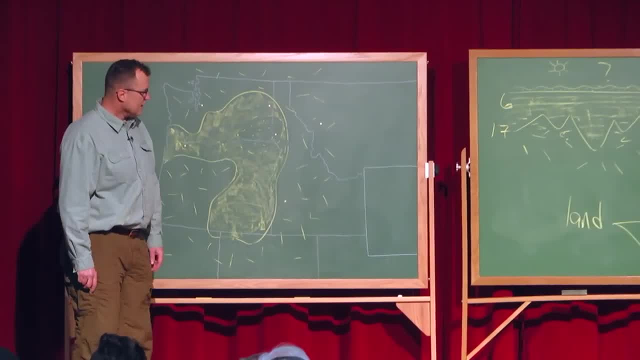 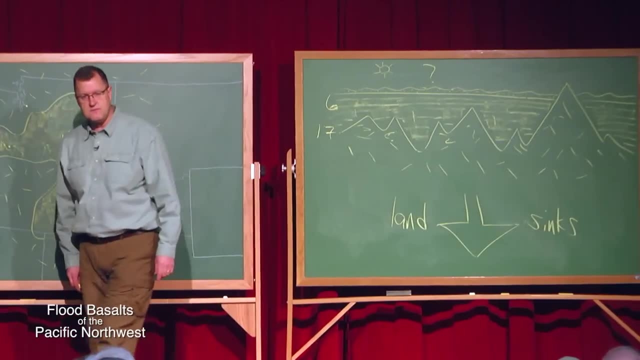 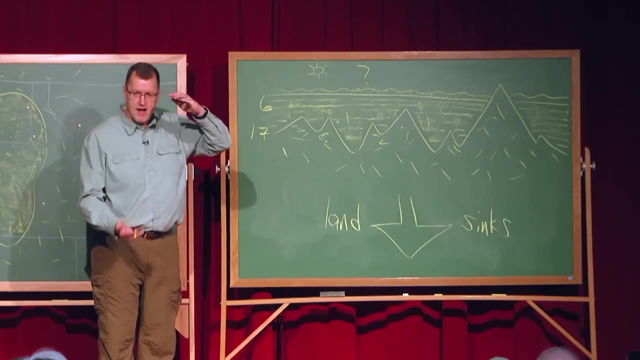 It's been called the Palouse Problem for more than a century in geology circles. I don't know if you can read this from the back, but this says land sinks. How much weight are we talking about If we're going to erupt two miles worth of German chocolate cake? 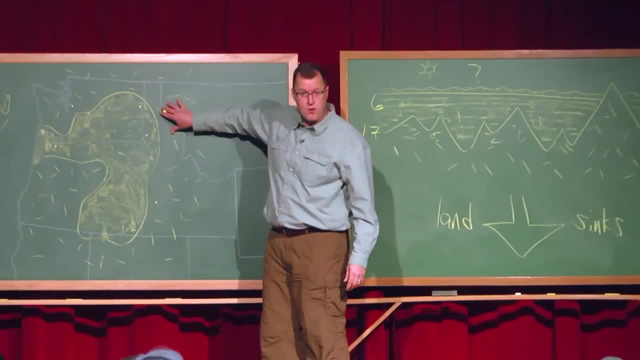 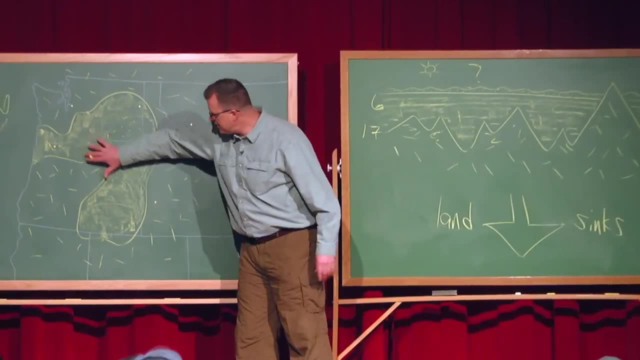 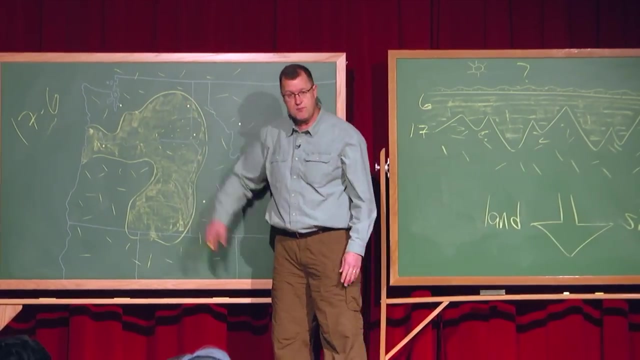 and plop it onto this landscape before 17 million years ago? The answer is a lot. It's going to weigh a lot And we are sure that this portion of the Northwest has been physically depressed. We have crustally loaded this section of North America, excuse me, Pacific Northwest. 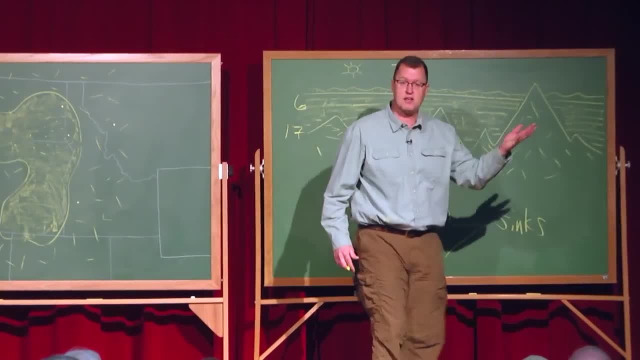 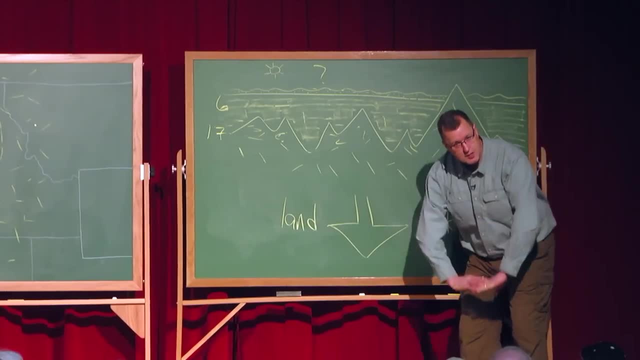 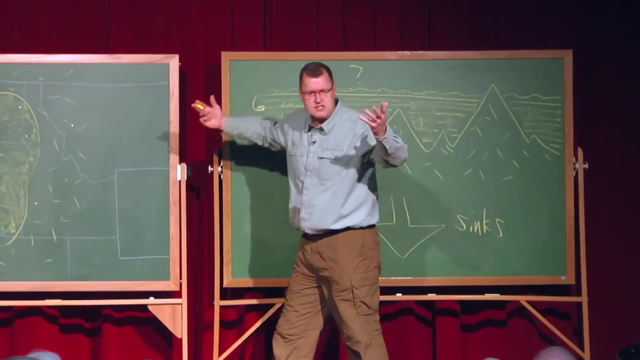 with these thick lobs. We do this with ice sheets, but the ice eventually melts away and the crust rebounds. This is permanently displaced, Permanently depressed, Downwarped And elevation of what The Tri-Cities is 500 feet above sea level or something like that. 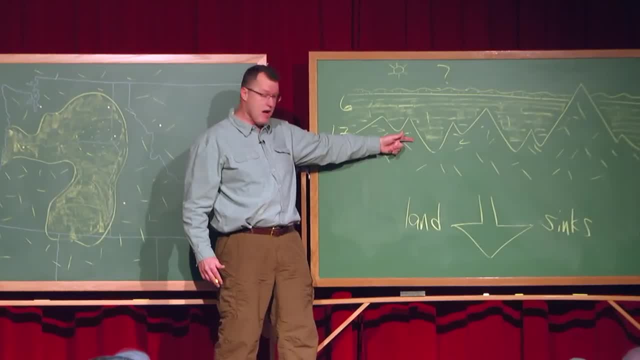 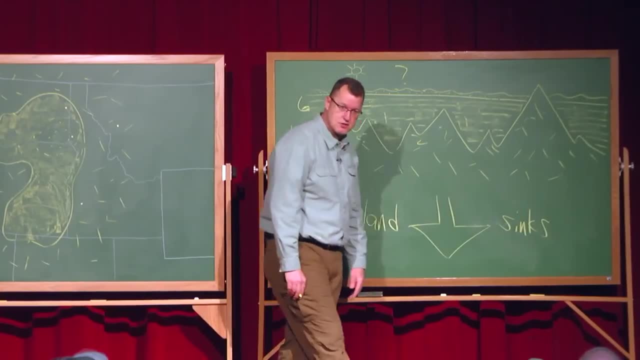 This is a landscape that was at sea level or higher. These are mountains that are now more than 10,000 feet below sea level. That's how much crustal loading or sinking we're talking about. So the mantle, which is below sea level. 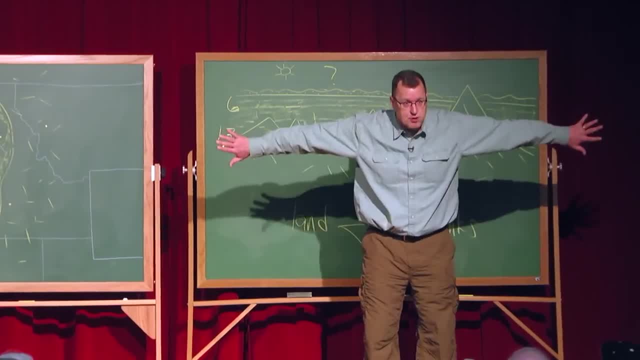 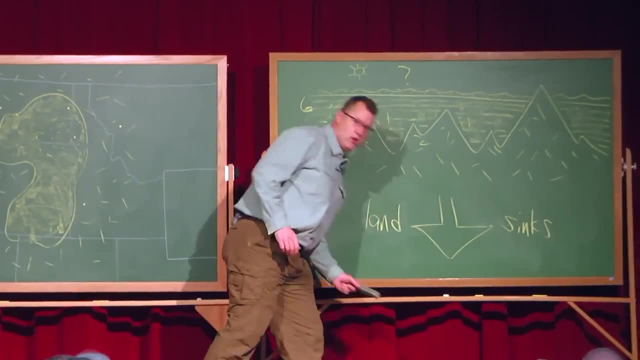 The mantle which is below the Earth's crust must have been displaced or flowed away from this subsided region. Okay, onward, Oh, you're like. well, can't we do a little question and answer here? No, there's 250 people here. 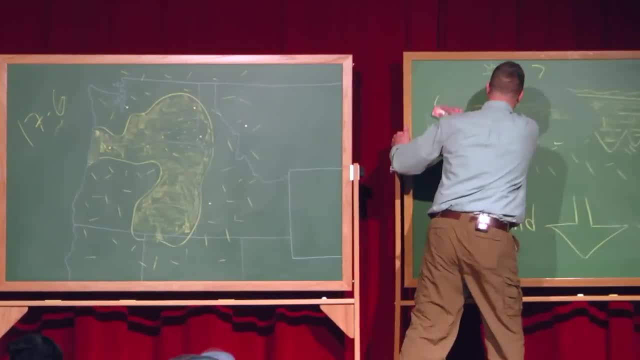 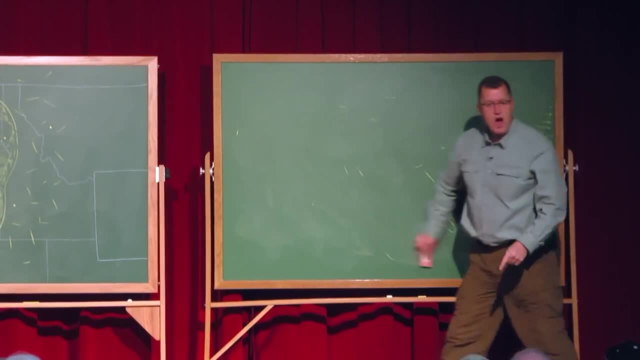 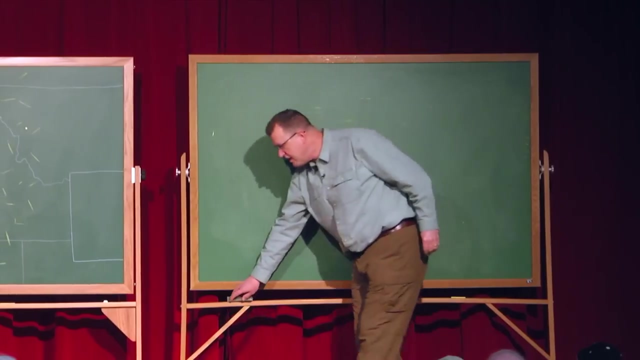 We can't do that, Okay, so we're moving on, We're keeping it going. So let's take that German chocolate cake, which again is our stack of lavas. By the way, there are 300 separate lavas. Did I say that already? 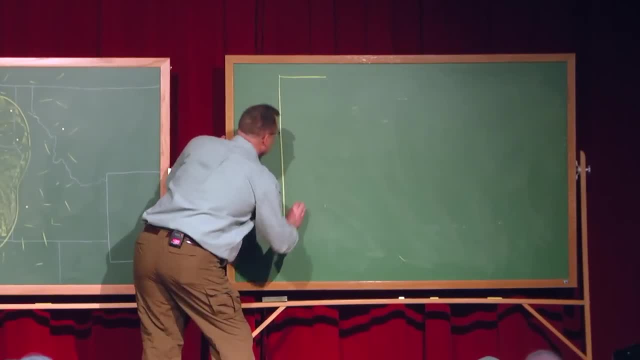 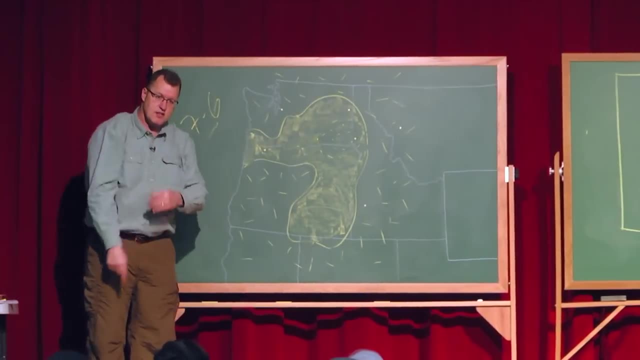 Maybe, maybe not. Let's do a little stratigraphic column. Let's basically go through our cake from bottom to top. We're drilling down into these lavas now And I'm not going to go through all the literature and all the names and all that sort of stuff. 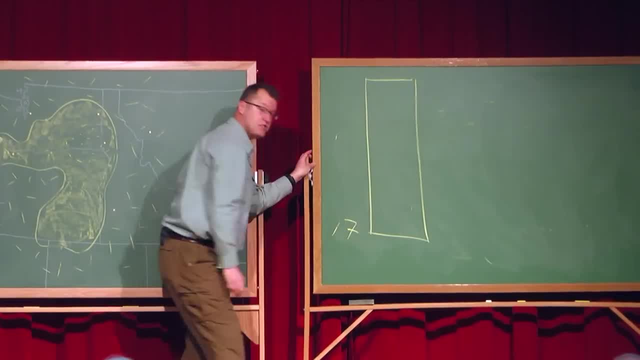 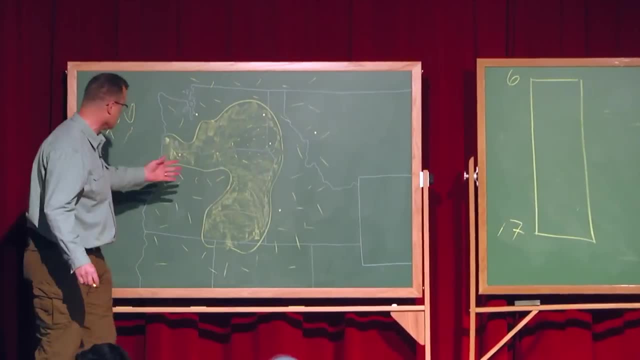 I've done that work for you. But down here at the bottom, here's 17 million years ago. Here's 6 million years up here. Now, that's a misleading way to say this. Technically, that's true. These lavas came out 17 to 6 million years ago. 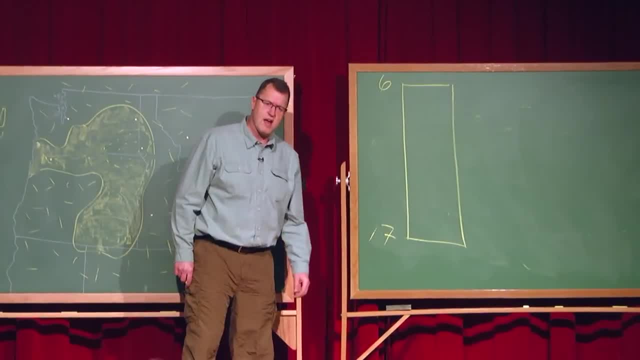 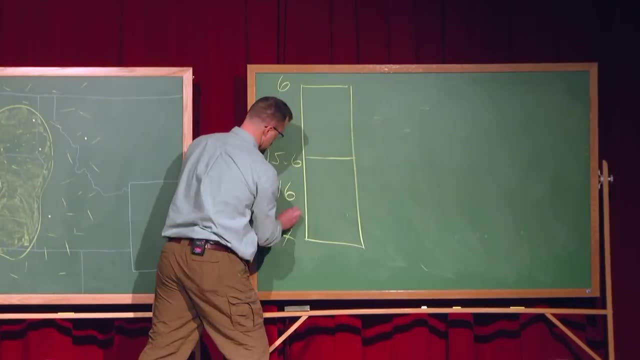 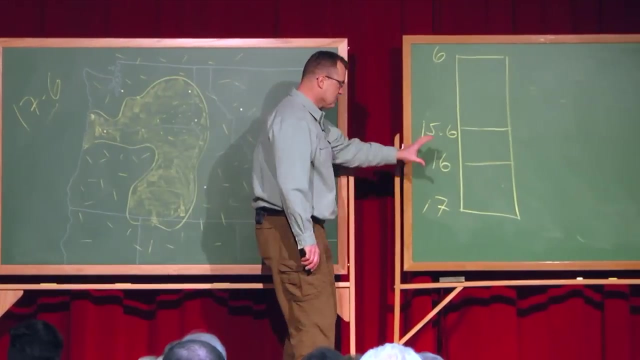 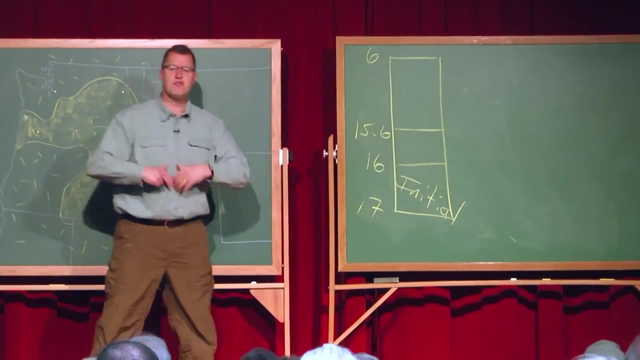 But, as we'll see here, it's not the best way to portray what we're talking about. 16, 15.6.. We can really subdivide these eruptions of these basaltic lavas into sub-events. We have kind of an initial phase, an initial phase of the eruption. 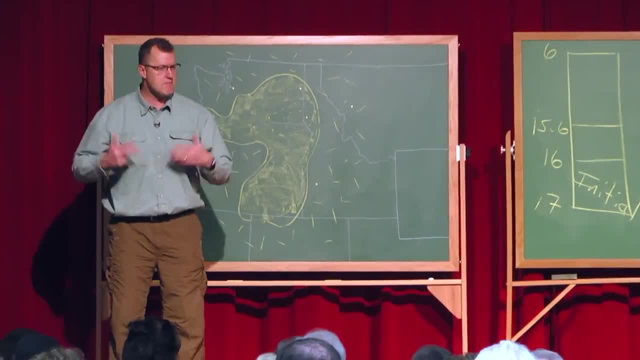 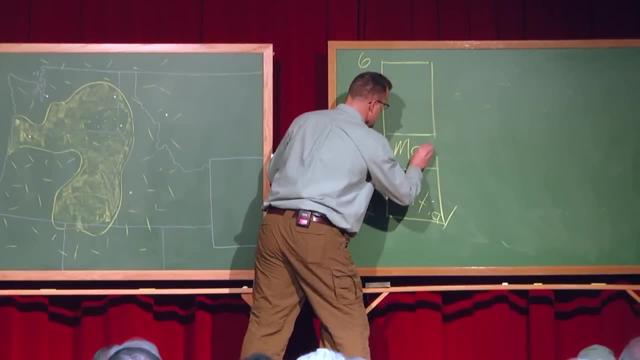 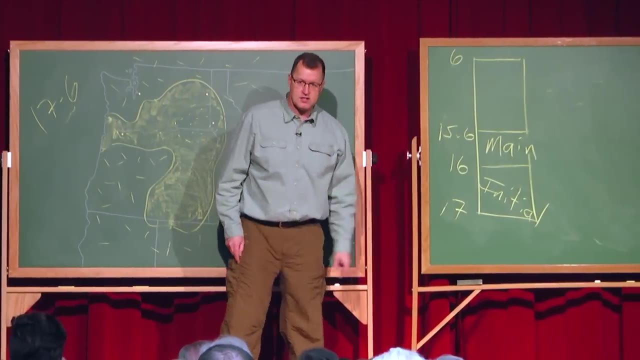 The first 1 million years are relatively minor lavas coming to the surface- There's a payoff for this discussion, by the way, coming in just a second- And then we have a main phase where the system is really working full throttle And notice that's just 400,000 years just. 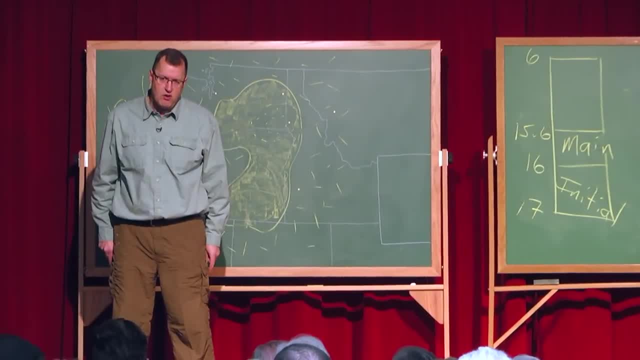 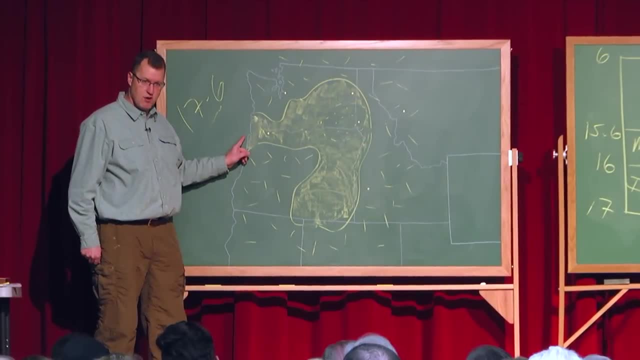 It's a relatively tight window where we're really pumping out these lavas, And these lavas are literally coming out of the ground in Idaho and flowing to the Oregon coast. It's just during that main phase time And then this waning phase. 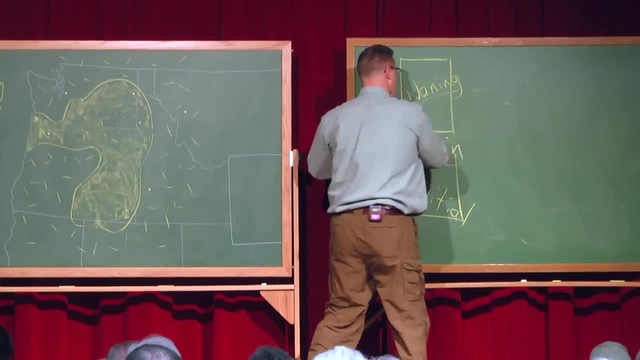 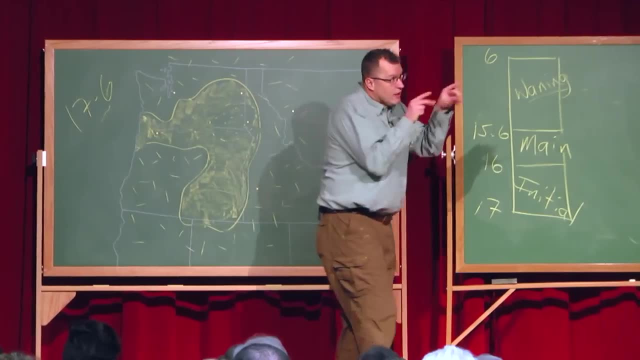 These are not my words. These are from some of the geologists who have been working on this. The waning phase is more than 10 million years. There's minor little drips and drabs and little worms of little orange things coming out just on occasion. 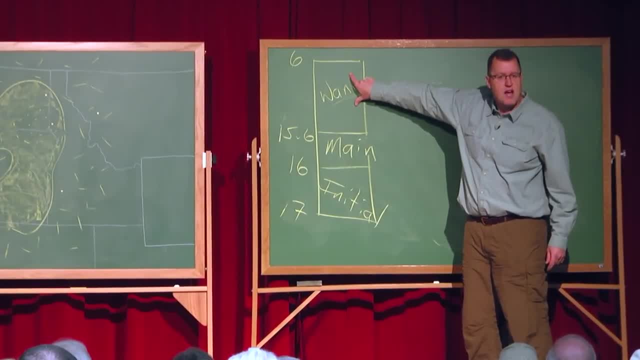 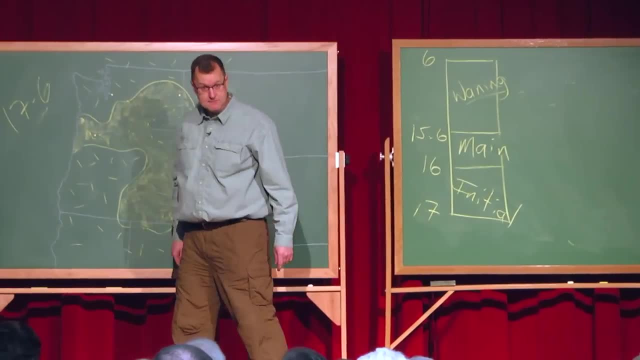 But this thing has finished with a whimper. It has not finished with a bang. We'll talk about some of these waning phase lavas because they are most prominent in Washington: The Ginkgo lava flow, The Rosa lava flow. Maybe some of you know some of those names. 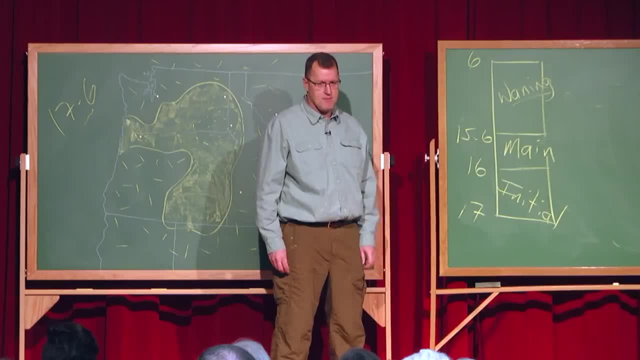 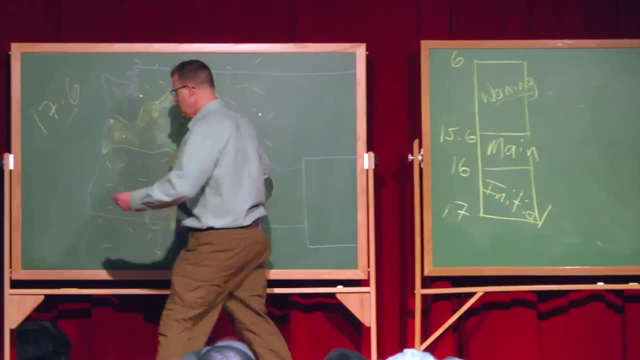 But this point of this stratigraphic column is to show that we've got a main phase right here. Okay, With this map. Hey, you want to see a magic trick? I got an eraser. I only got one eraser up here. 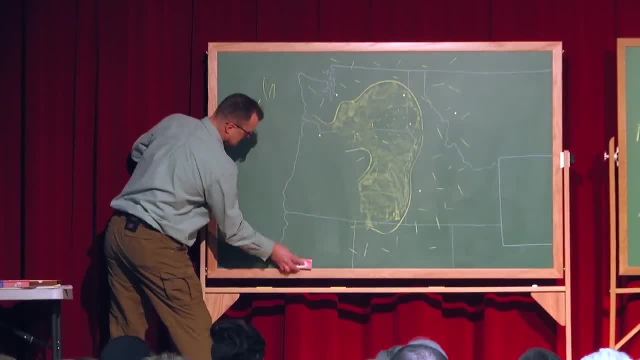 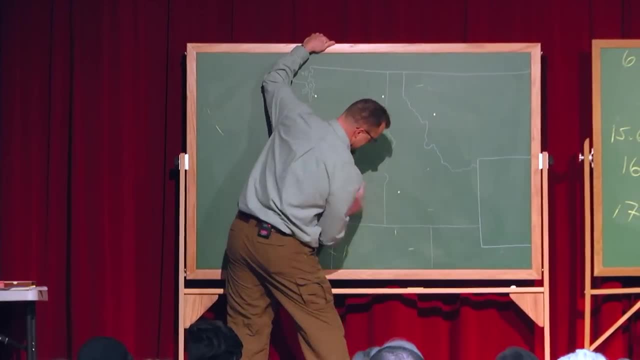 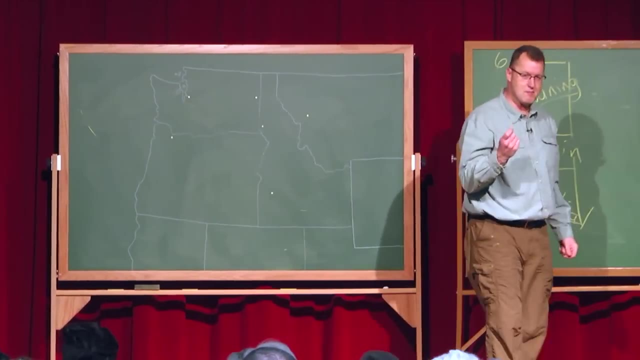 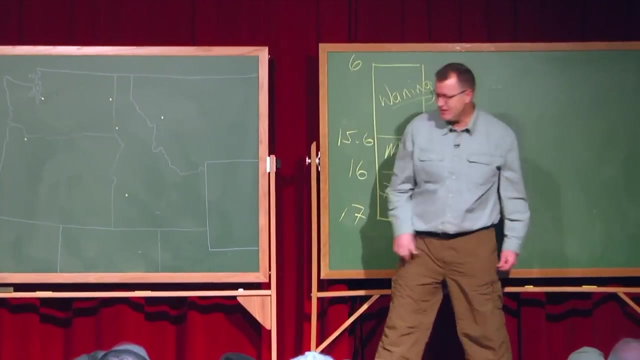 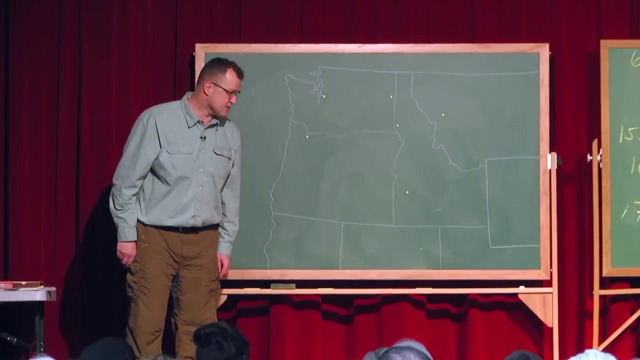 You ready, Turns out. Sharpie markers also have Sharpie markers. with paint, It's like a paint can. So Okay, Why 17 million? And where are these lavas coming from precisely? There's a relationship with these lavas to the Yellowstone hotspot. 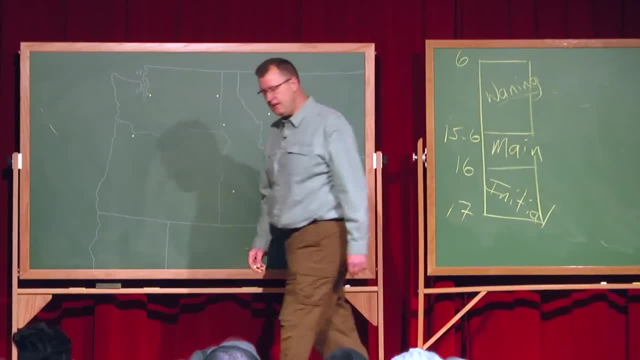 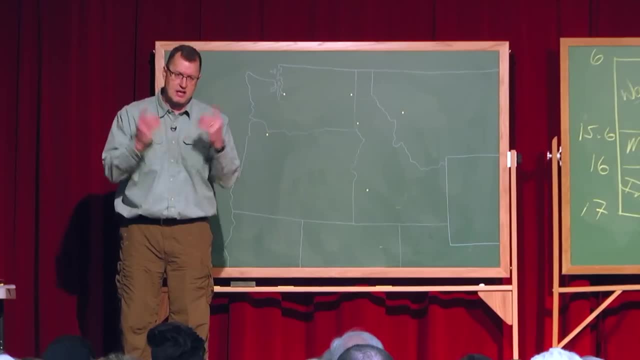 With the Yellowstone hotspot. So let's fill you in. And there are some problems with this connection. Not every geologist loves this idea, But I'm a fan And many people see at least a timing connection And that's what we want to try to do. 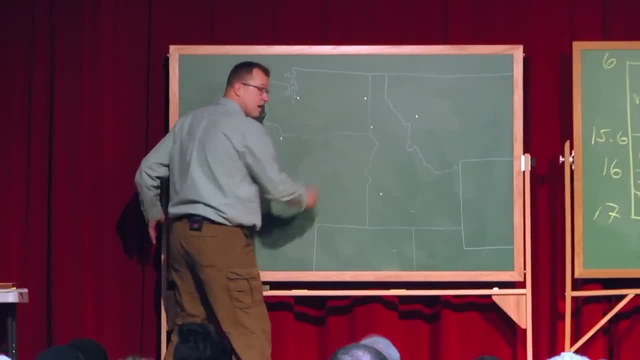 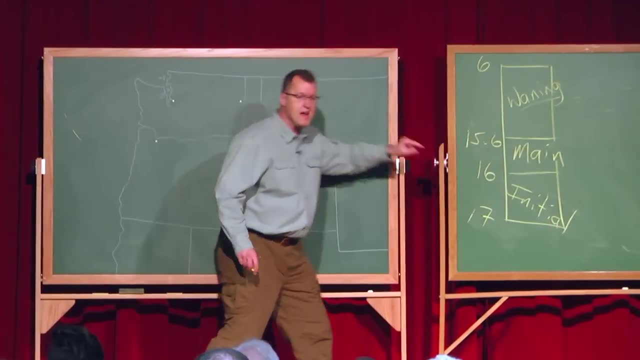 So where are these lavas? The lavas are here. They came out of cracks. Sure, Where are the cracks? Well, the waning, Let's do it, Let's go backwards. The waning phase cracks, as we'll see with these beautiful maps I have for you, are generally up here in southeastern Washington. 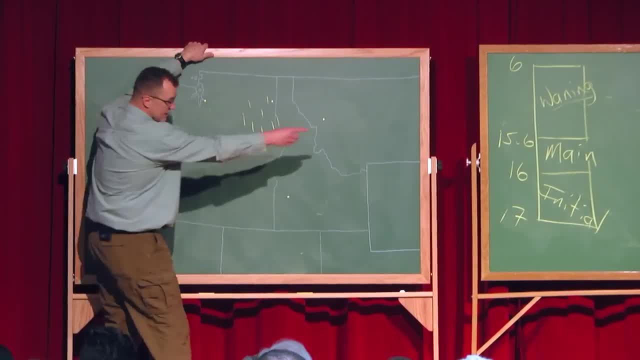 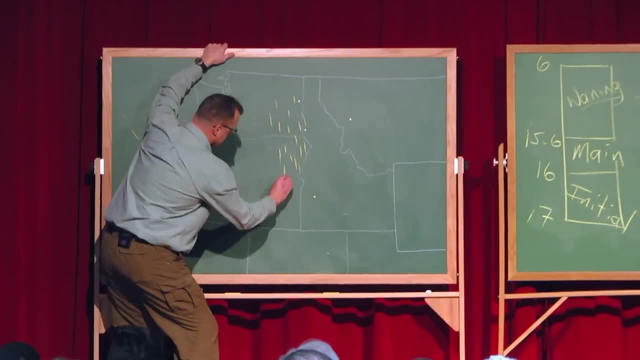 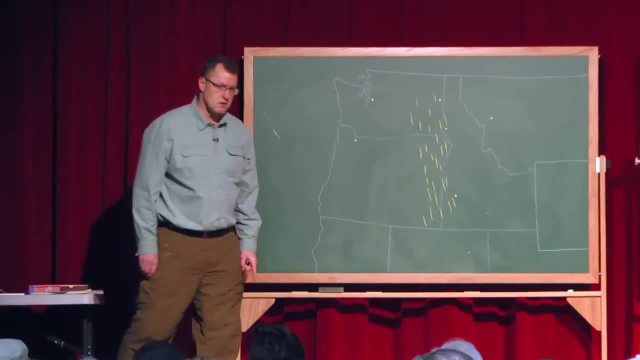 The ones that are young. Let's go back in time, During the main phase. the cracks are here. During the initial phase, in other words, when this system got started, the cracks were down here in southeast Oregon. So we're not making a cake and we're not having the lavas come up each and fill the same cake every time. 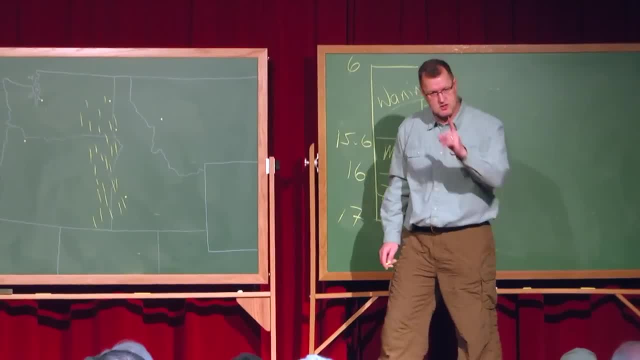 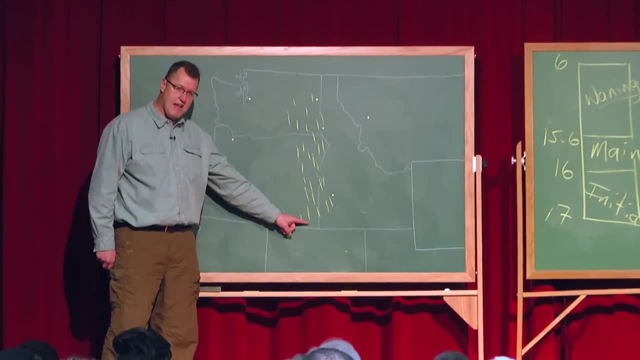 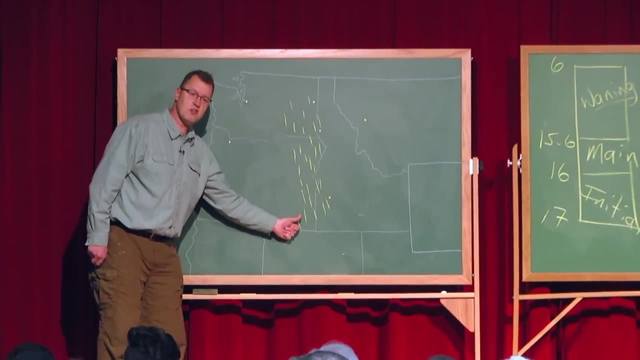 There's portions of the cake we're building geographically at different times. Here's the point: This whole volcanism story to make this German chocolate cake is starting down here, And these cracks are getting younger as we go north. Something is happening initially here and by the time we're done, the cracks are opening up here in Washington. 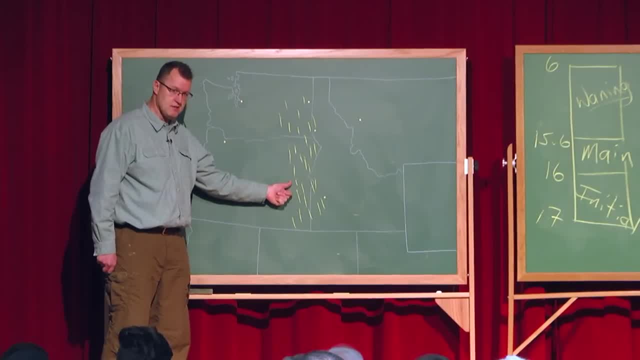 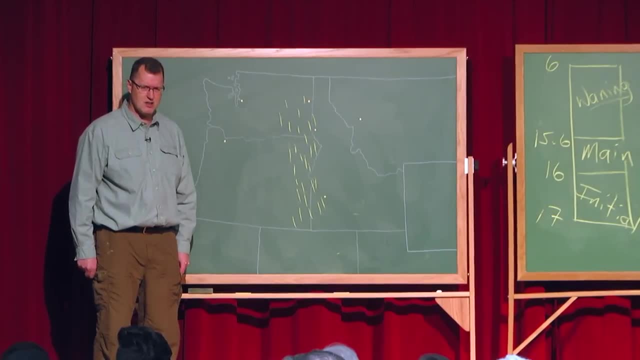 That's the convincing evidence. All these cracks are not the same age. That's the convincing evidence that it's related to the Yellowstone hot spot. And you're like what Yellowstone? Is that like Wyoming? Yes, Yellowstone is right here. 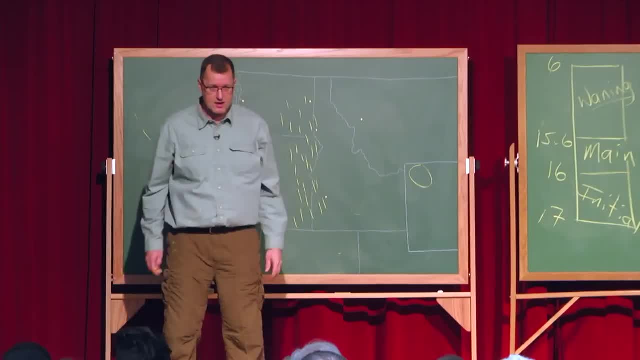 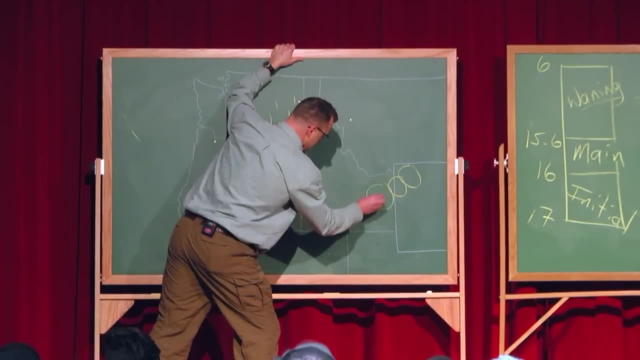 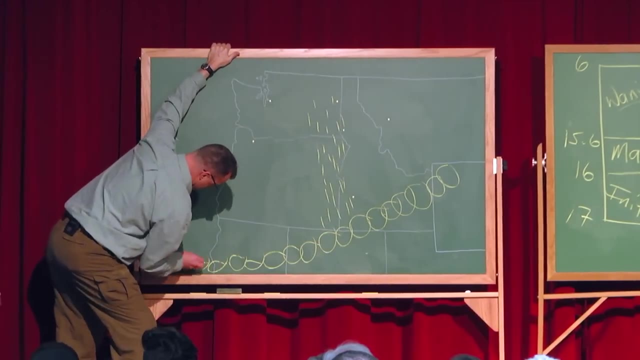 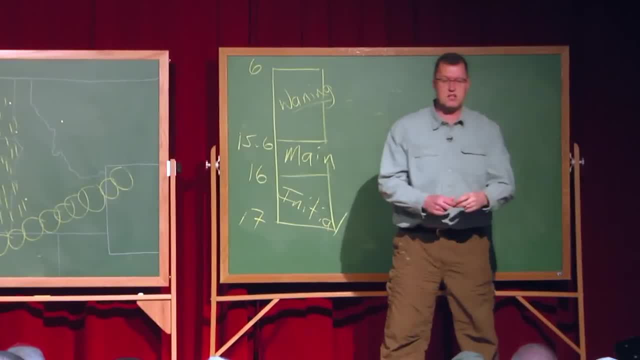 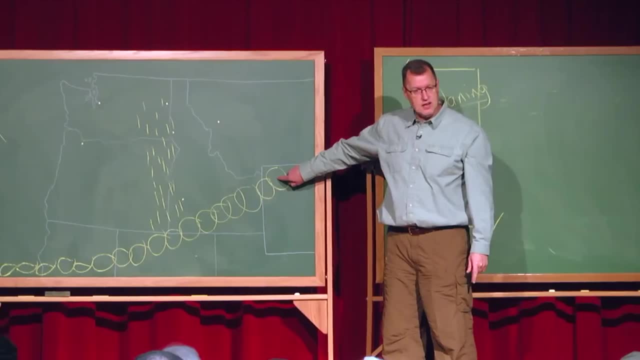 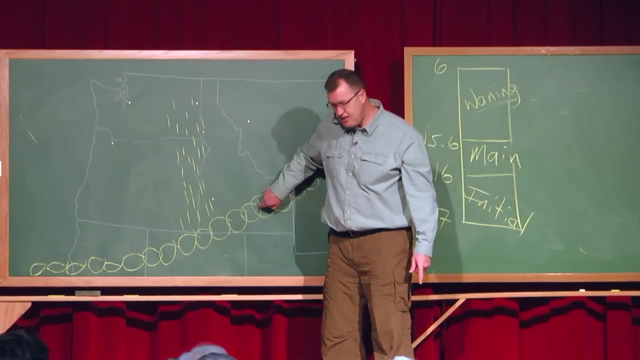 Each of these is a circular caldera, Each is from an explosive volcanic activity And each of these is a very specific activity related to the Yellowstone hot spot. The concept is: today there's a Yellowstone hot spot beneath northwestern Wyoming, But in the past the Yellowstone hot spot was at different locations. 5 million years ago the hot spot was at Pocatello, Idaho. 10 million years. it was at Twin Falls, Idaho, 17 million years ago. where was the Yellowstone hot spot? Right here in northern Nevada, where we have our earliest cracks forming? 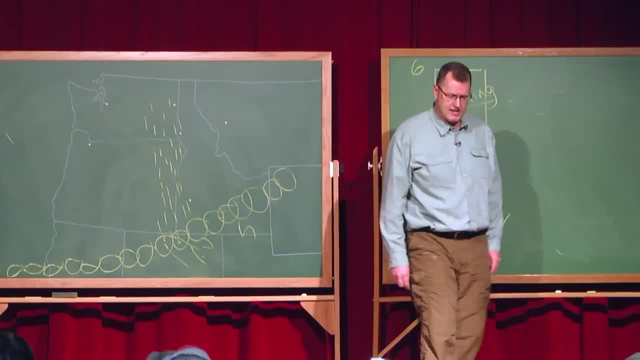 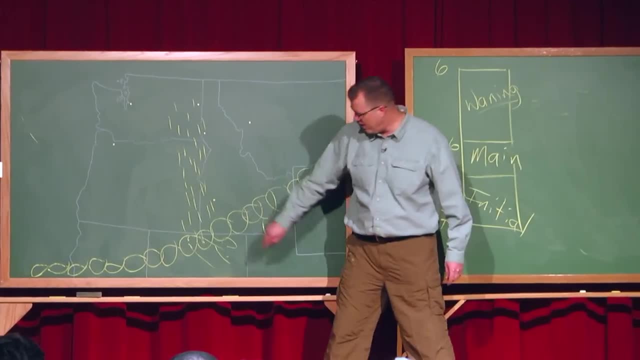 cracks forming at the same time. Is that a coincidence? You can't tell me it's a coincidence. You can't tell me. the cracks that are making our lavas and this Yellowstone hotspot story happens to be at the same place, at the same time. 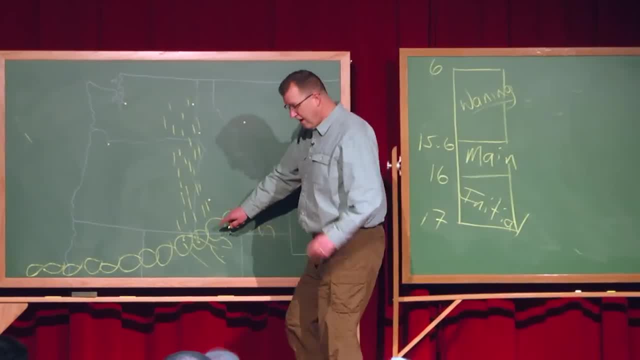 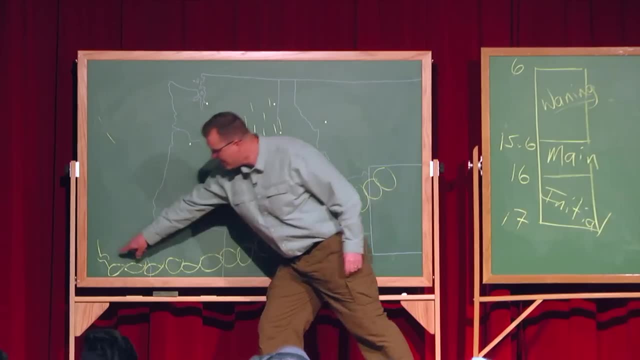 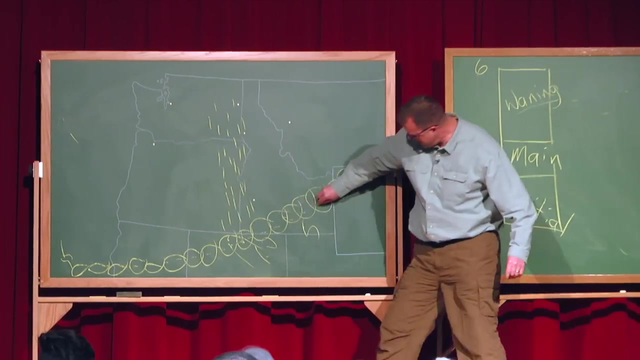 without any connection whatsoever. By the way. last winter we had a lecture talking about evidence for the Yellowstone hotspot being 55 million years old. at least 55. And you go. the hotspot then is moving: 55,, 40,, 30,, 20,, 10. here Some of you. 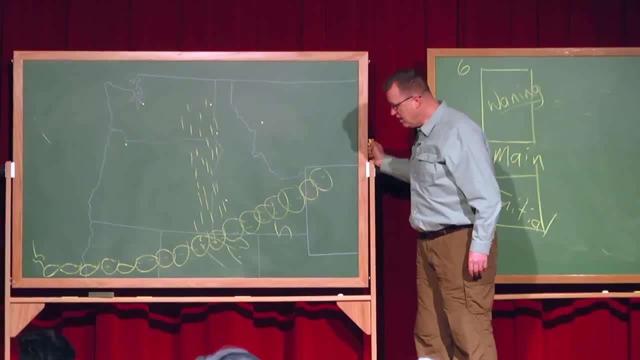 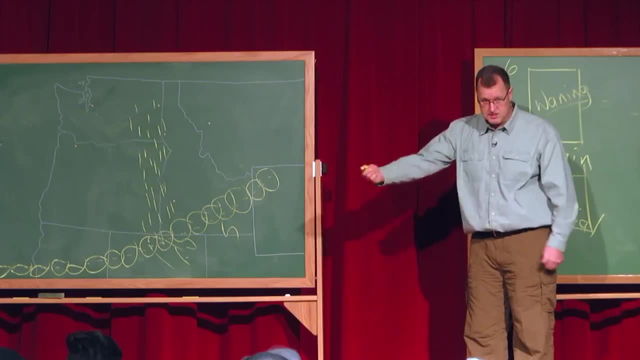 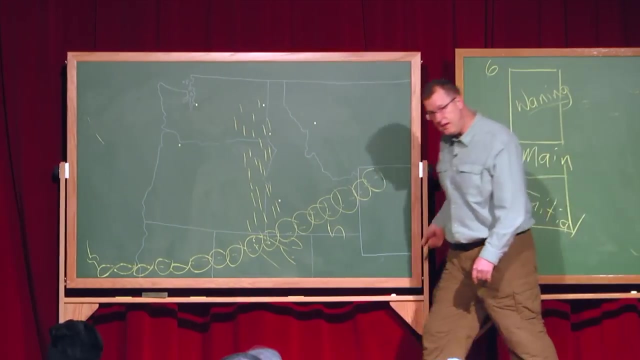 know this. The hotspot is not moving. The North American plate is moving over the stationary hotspot. We can still get the same pattern right: Instead of moving the heat source, we're holding the heat source steady and we're moving the North American plate over the top. Regardless, all I'm trying to say is that 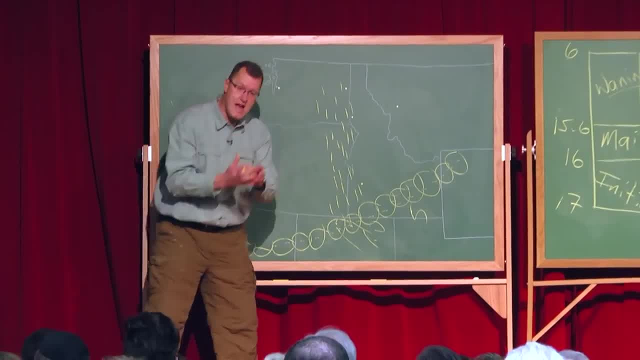 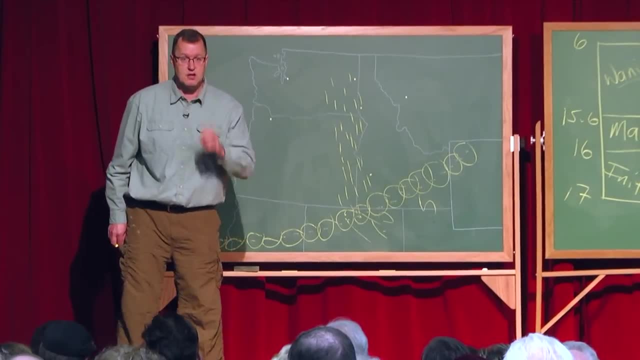 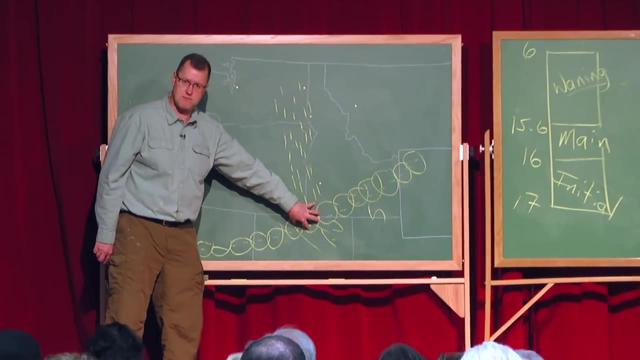 the. there are temporal and spatial connections between the Yellowstone hotspot story and these cracks. I'll give you one example of what's a problem with this. Why would the main phase be up here? when we initiate the story down here, Wouldn't you expect the biggest and most voluminous lavas to come out where? 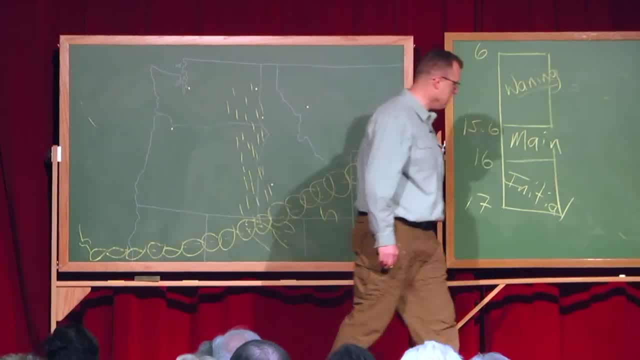 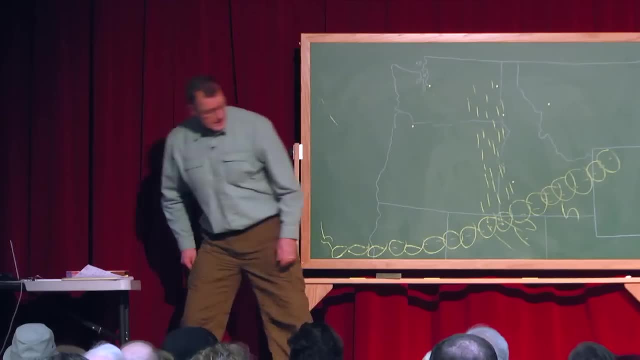 we have the heat, You get it. So there's a lot of back and forth, But Yellowstone hotspot is a story that I like. We're keeping it moving. We're keeping it moving. Where's my little sketch here? Hang on just a sec. 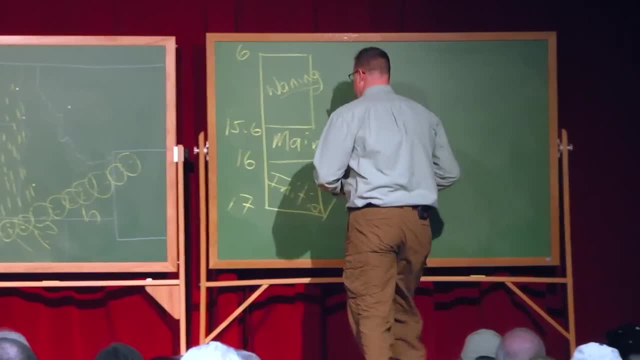 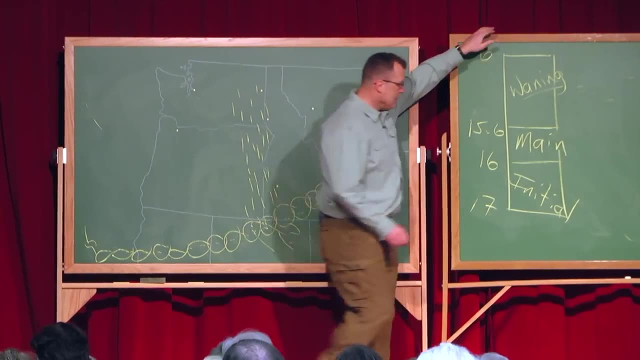 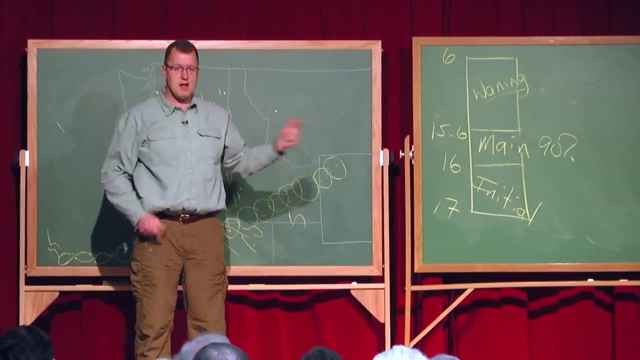 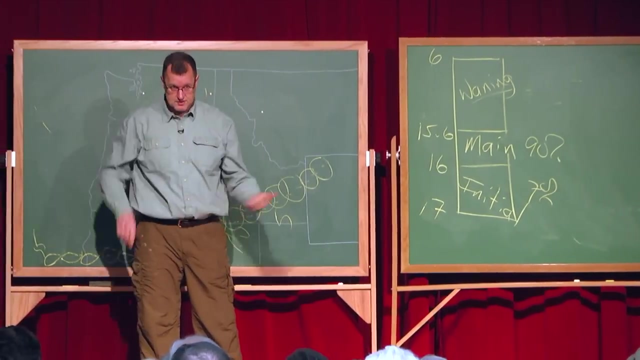 Right, right, right. One more thing. So the whole cake was not built steadily. as I've already implied, 90% of the volume, 90% of the magma that came to the surface came out during that 400,000 year old time. Only 7% of the Columbia River Basalt flood province came out early. 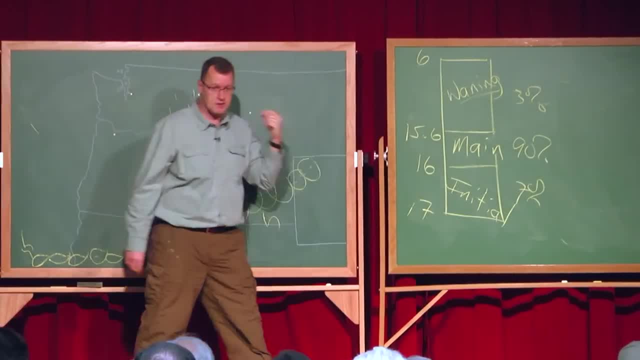 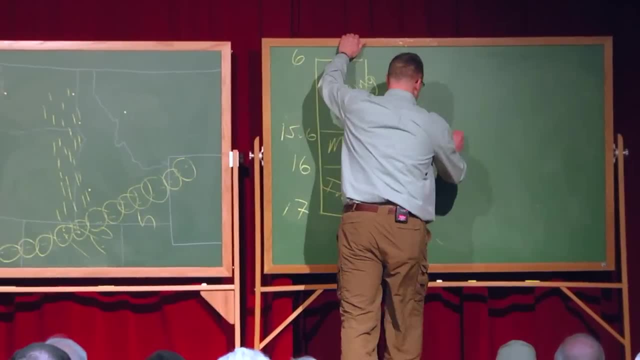 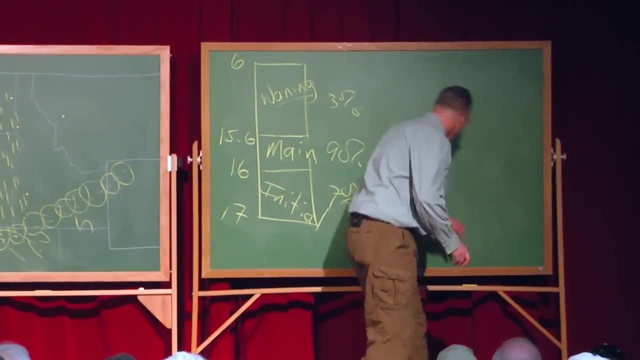 And only 3% of the total volume came out in the last 10 million years and change If you're a numbers person and love the number of flows. we're talking roughly 180 separate basalt flows during the main time, 100 flows roughly in this waning time and 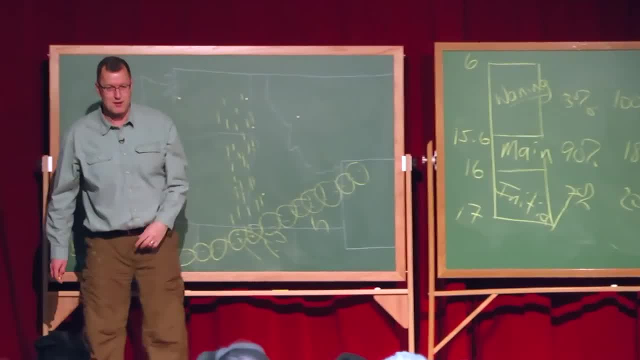 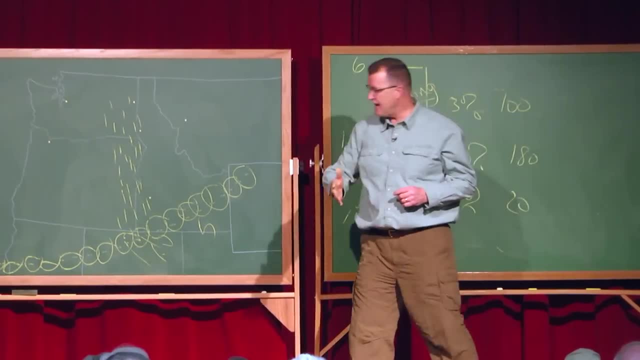 20 flows initially. Hopefully, my math adds up to 300.. Okay, Good, I want to do a couple more things with these chalkboards, and then we've got to go to these places. I've got specific directions for you. That's maybe the thing. 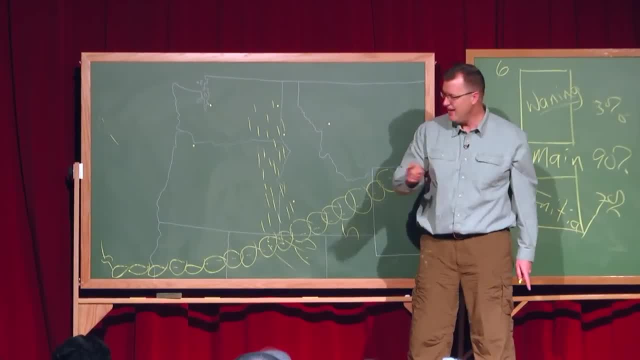 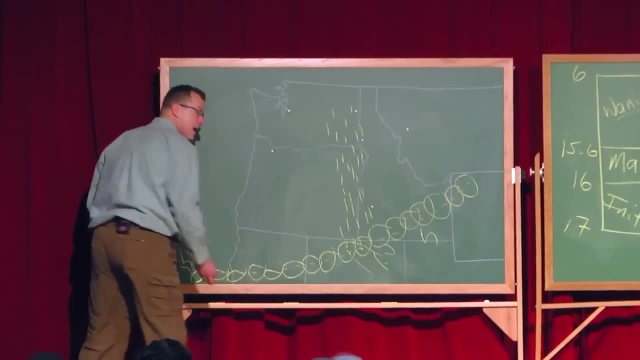 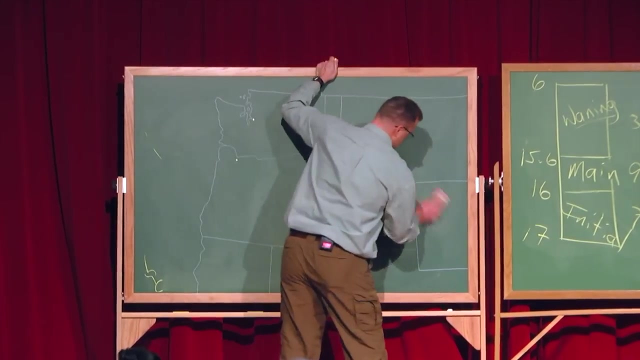 I'm most excited about tonight: Specific driving directions on how to get to some of these cracks, How to know you're at ground zero for some of these eruptions. That's what we're going to do right now. Oh, there's murmuring in the crowd. You like that? Alright, So here. 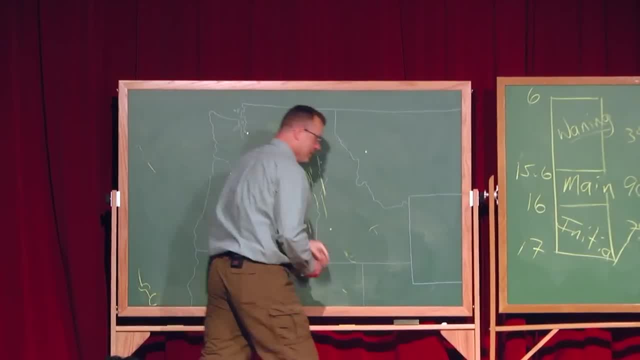 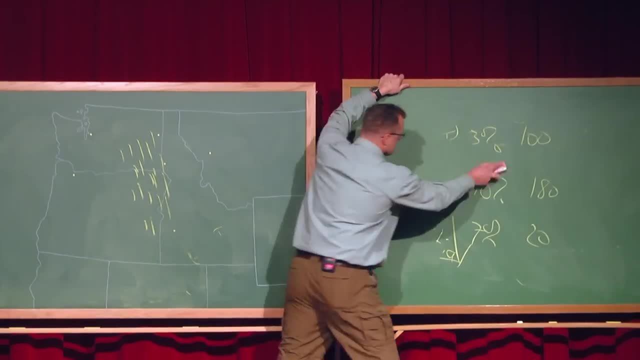 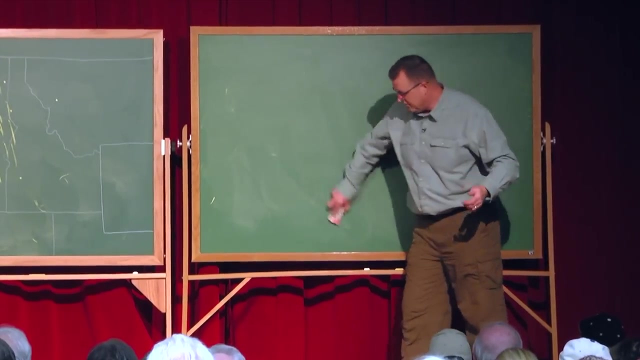 are the cracks. We know they're not all the same age right Now. I've been here 25 years, been teaching about these lavas for 25 years, So I have a standard approach that needs updating. That's why we're doing this lecture. 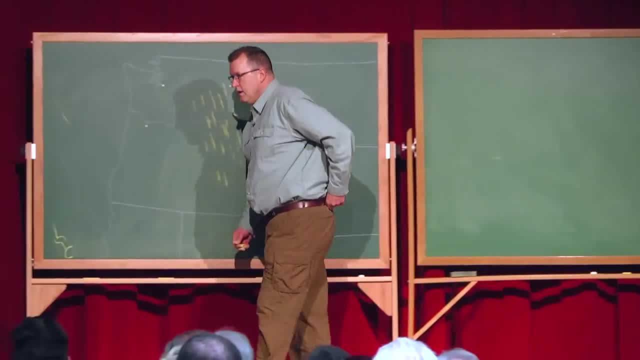 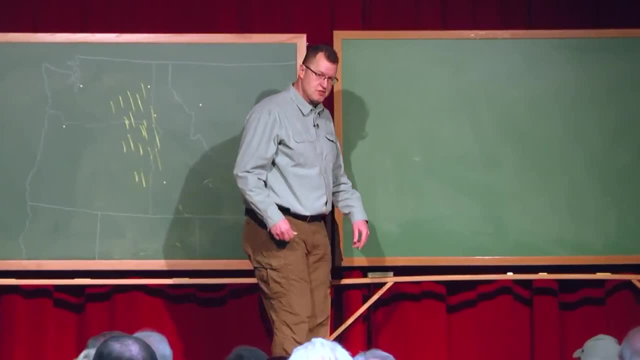 I'm kind of bored with it. It's kind of stale. So here's one thing that I had no idea about until two years ago, And I got so excited that I spent much of a summer out there playing around with this discovery. I didn't make the discovery. 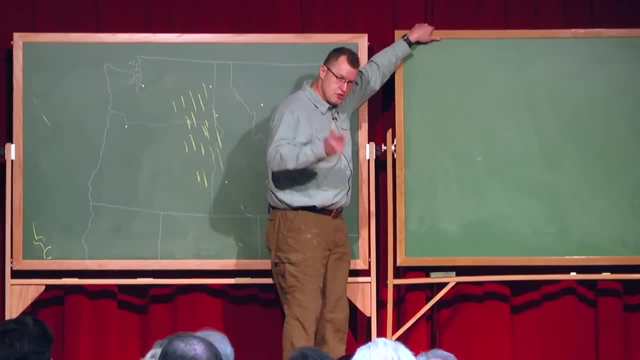 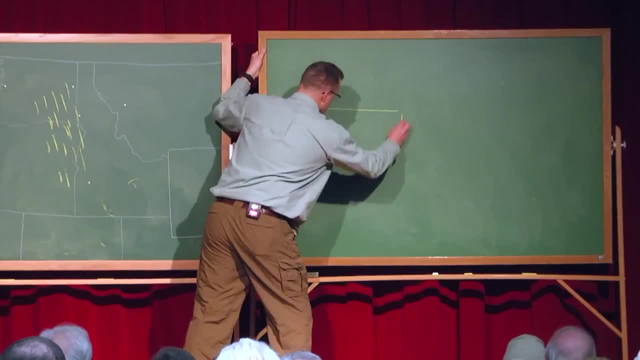 I have people who help me find new scientific papers. John Lash or other folks send me good information and I just follow those sorts of things. So for 25 years I would say: hey, students at Central, you want to go find these cracks? 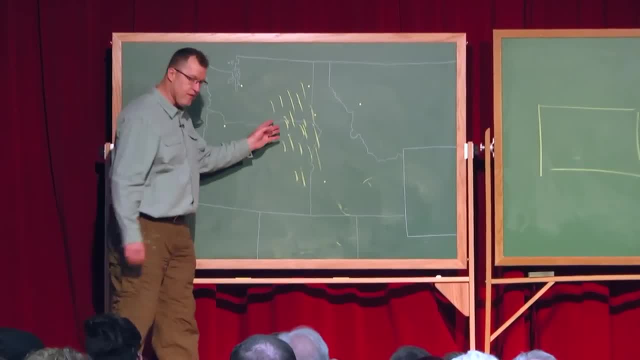 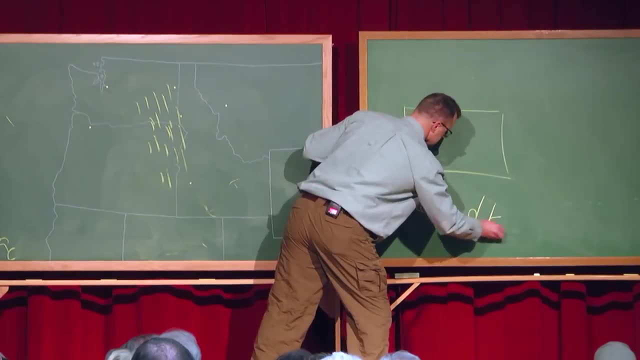 These are called fissures. That's where the lava came up. You want to go find a fissure? You've got to go find what we call a feeder dike And geology as a dike is typically a vertical wall. Here's a friend named Tom Tabard who And this last little guy, just a little blip, coming up right at Tri-Cities. Good, So let's go to actual places where we can see some of those sources. Let's do this, Let's do this again. Yeah, yeah, yeah, yeah, yeah. And now Grand Ronde. this is the main phase. How can we find those feeder dikes? Well, one way we can do it is to go to the Wallowa Mountains. Have you been? This is down by Joseph and Enterprise. That's one way to approach The Wallowa Mountains in the Wallowa-Whitman National Forest is mostly light-colored rock. The mountain range is mostly granite and limestone- light-colored stuff- And it makes it easy then To find our feeder dikes, because our feeder dikes are brown right. 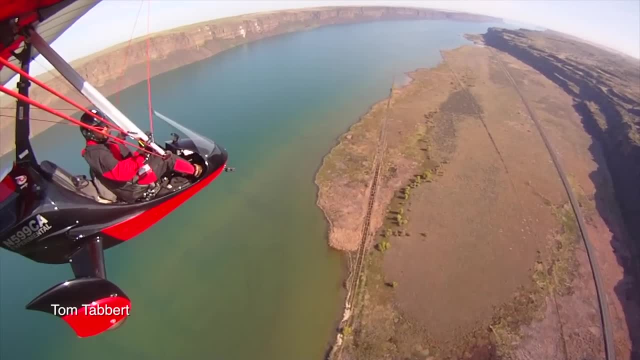 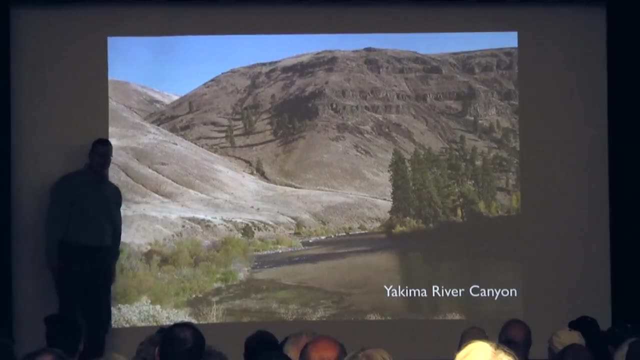 We can find those squirts of lava coming up through, And during the main phase we had that. This was all underground, of course, at the time, But we can find these feeder dikes. This is all, Andy Minor helping me out. 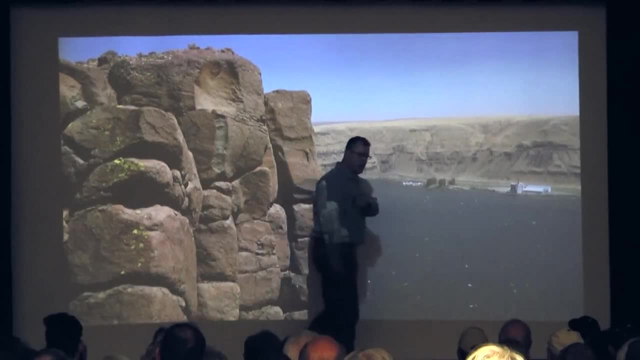 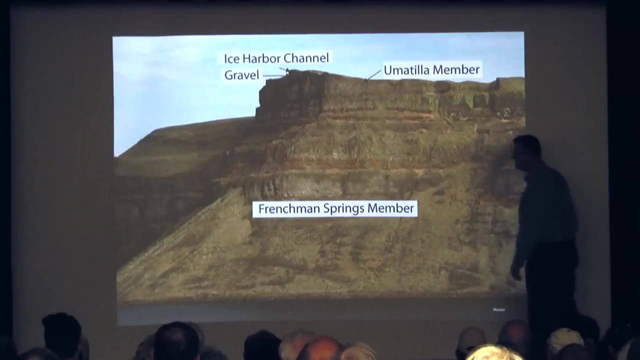 Feeder dike just sticking out like a stegosaurus plate. We did a backcountry trip this summer in the mountains. I knew I was doing this lecture, so we were on the hunt for these feeder dikes and they were pretty easy to find. 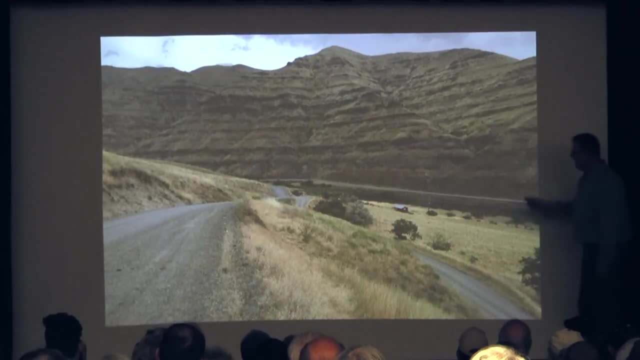 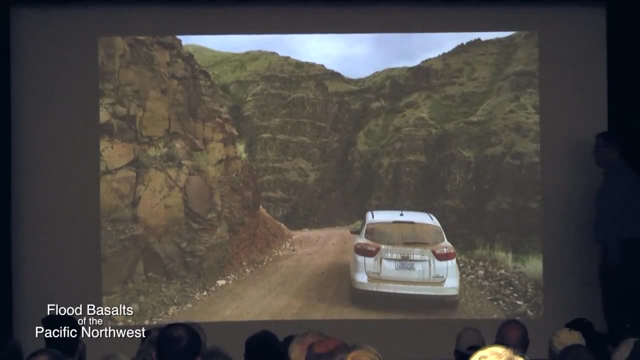 There's thousands of these feeder dikes. Each of the dikes are not very big. You're like, well, geez, that thing is going to feed a lava flow that goes all the way to the coast. No, But if you have a hundred of these feeder dikes all active at the same time, you can. 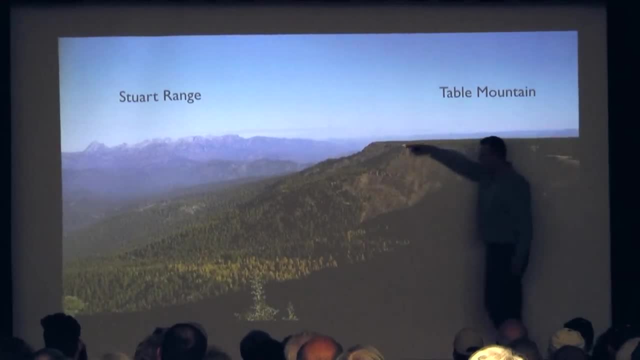 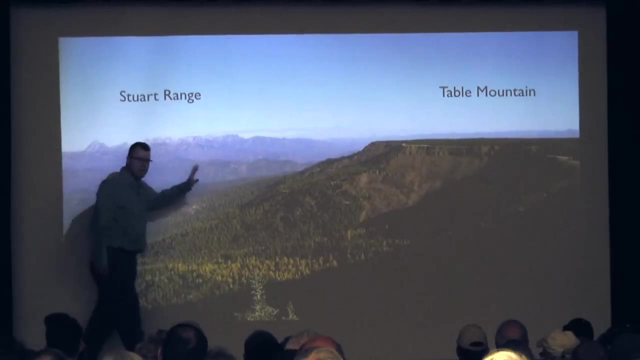 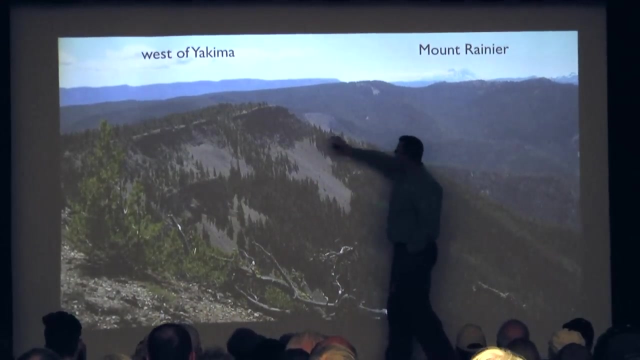 feed some pretty impressive lavas. So feeder dikes- there's one right here in the trees. We have video of a feeder dike, Yeah, OK, So there's a waterfall there because of the feeder dike making that vertical, There's a vertical resistant ledge. 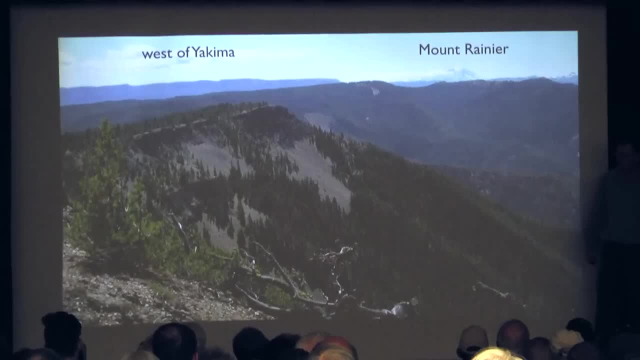 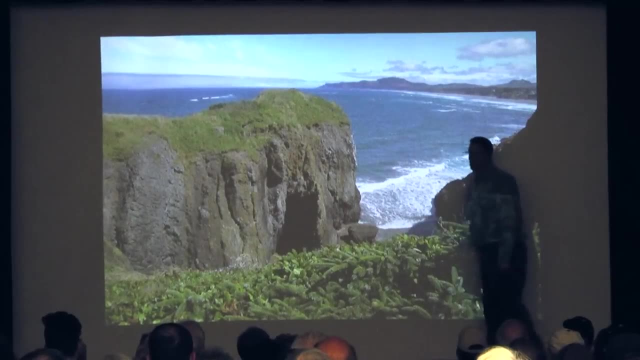 So all through the Wallauas, a lot of the main phase feeder dikes. Well, let's say you don't want to hike or you can't hike anymore. My knees are shot too. How about we drive? We go to the Grand Ronde River Canyon. So here's one of the best tips I've got for you. Have you been on this road? I hadn't been here until last summer. You go to Clarkston. Don't cross over to Lewiston, Fine town, I'm sure. 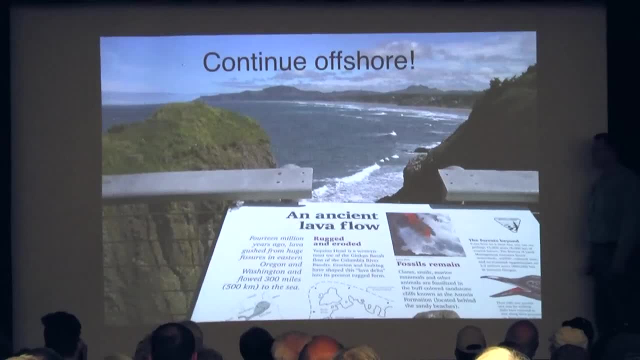 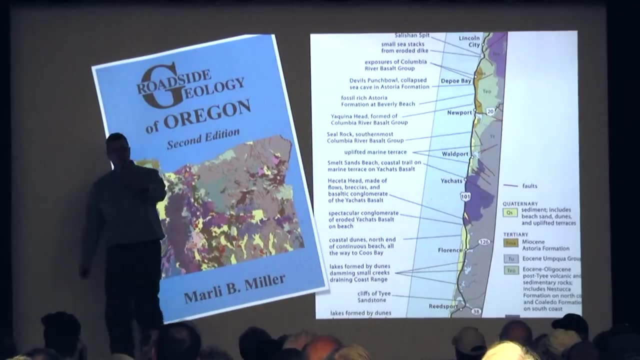 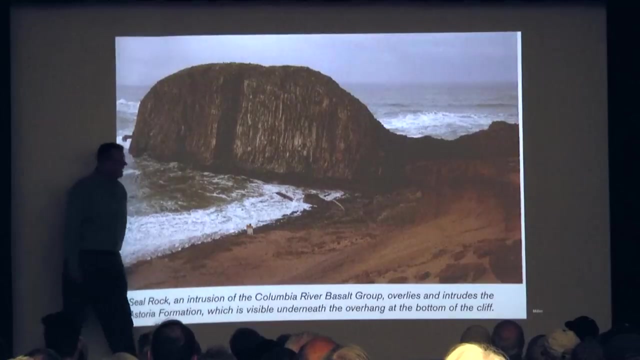 But stay in Clarkston on the Washington side State route, Washington State Route 129. A, Soton, Anatone, Field Springs State Park, and you're going to drop down to the Grand Ronde River Canyon. This is primo country or prime location for some of these beautiful feeder dikes. 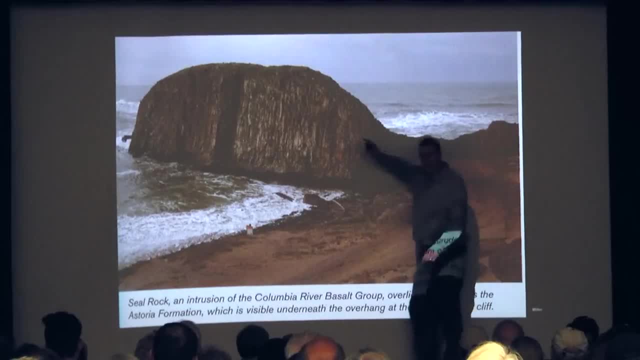 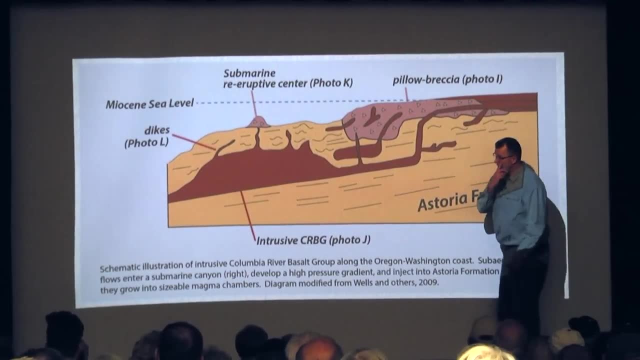 Each of these is a feeder dike from the Snake River all through the Grand Ronde River Canyon. And here's what they look. Look at this road, Putting this road in to get through this impressive German trail, And here's what they look. 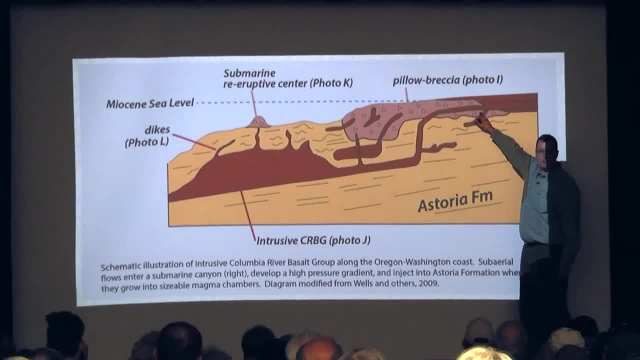 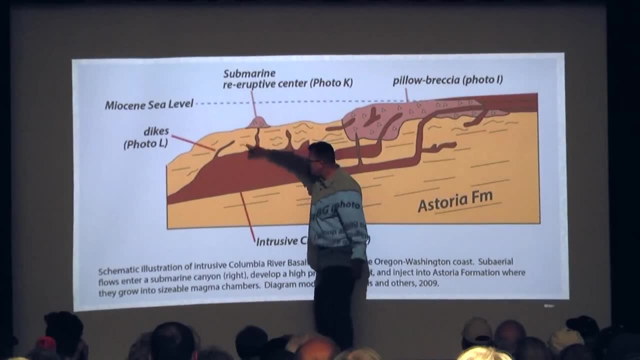 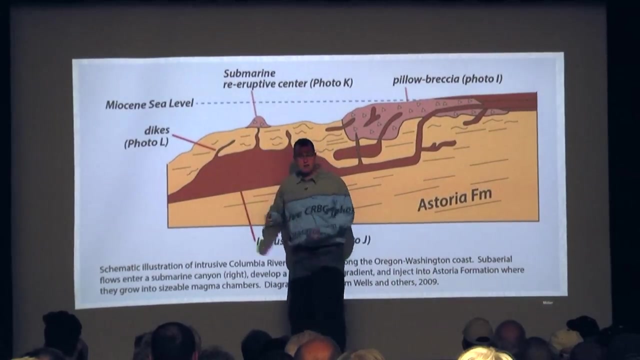 Look at this road. It's like a German chocolate cake: Layer after layer after layer. But once we get down to the river and we stop for some ice cream, can you see that something different is right here? It's a vertical layer of lava cutting across everything else. that's horizontal. 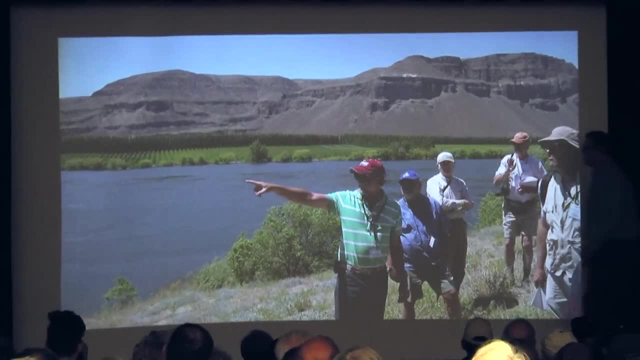 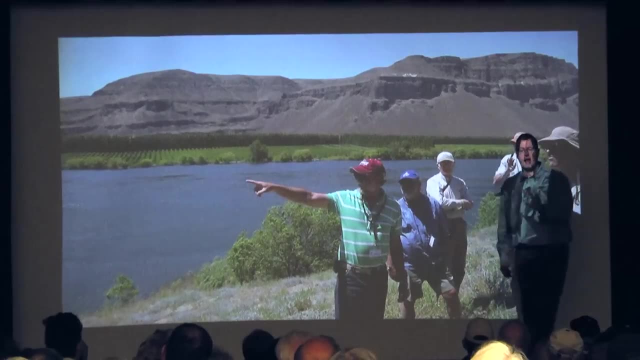 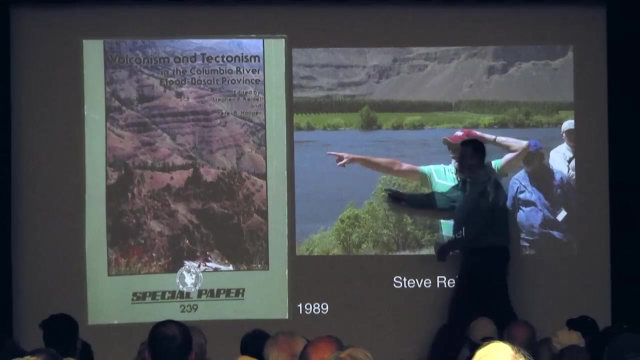 We're right here on the map, Vertical Cutting across horizontal. These are the feeder dikes that I have known about about for 20 years, But they're impressive and they are resistant. They stick out compared to the other parts of the cliff. It almost looks like firewood out behind your cabin. 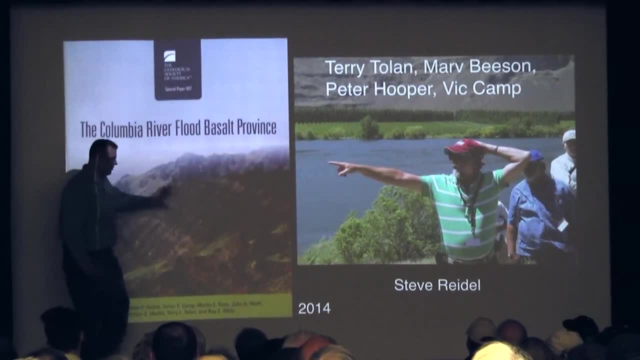 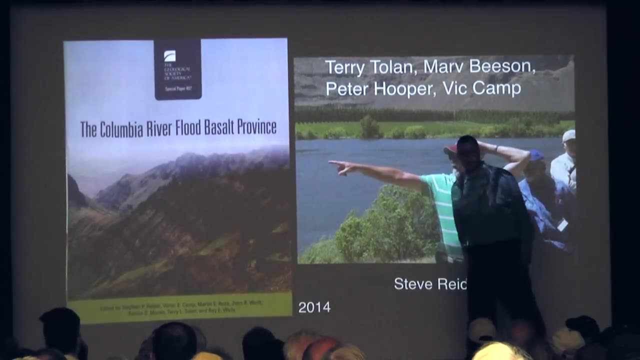 It's all stacked up like that. So Grand Ronde River Canyon, a beautiful spot. You can just hunt for these feeder dykes. They're all over the place if you have your eyes tuned for this sort of thing. Beautiful, The plumbing system of this fissure eruptions There's. 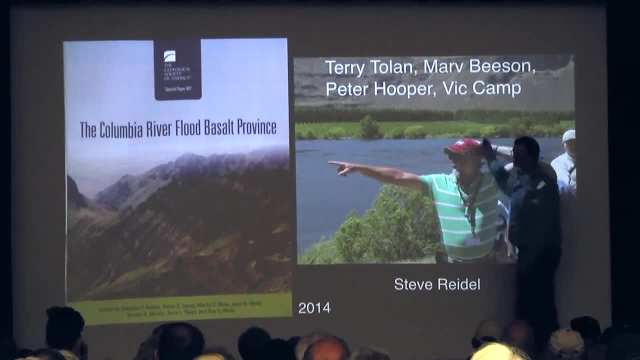 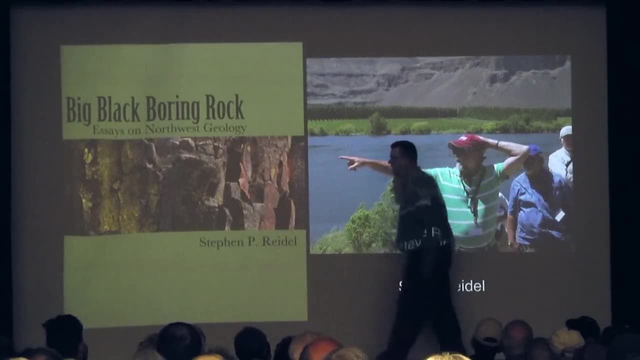 another one there, There's another one there. We got it right. So we're building to what We're building to the spatter. We want to go now to these newly discovered- at least to us- places where we can find where the lava came to the surface and fell out of the 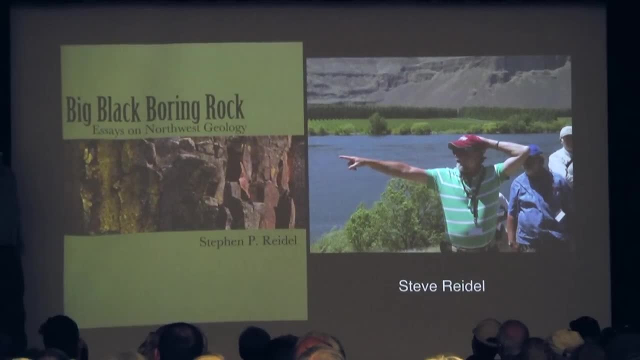 sky. I'm ahead of myself. We're still feeder dykes. I'm getting impatient. I hope nobody from Motorpool is here. You're not supposed to go off the pavement, but I guess I did All right. Good, We got it. We got it. We got a show of that little episode. These are five-minute episodes. 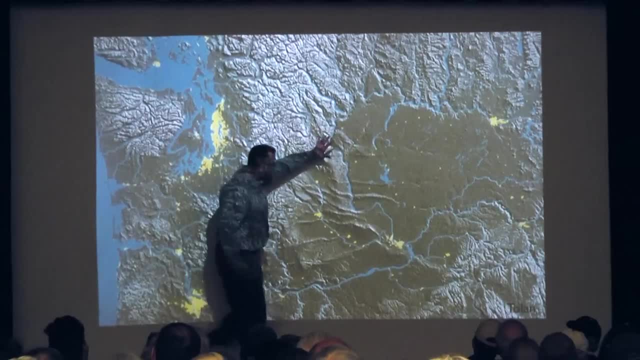 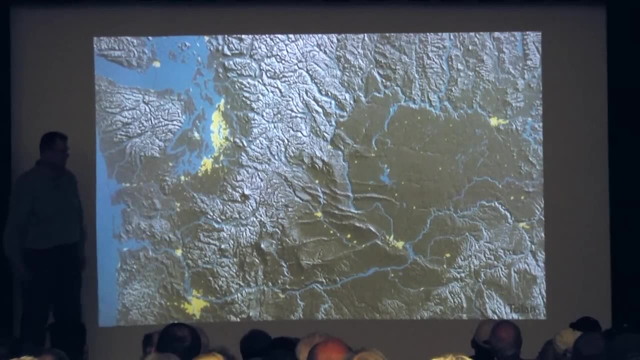 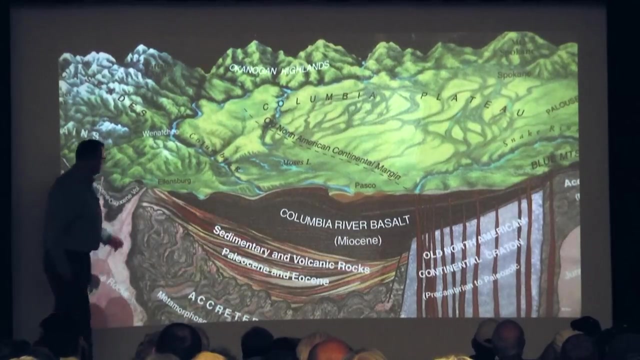 that are showing on PBS in Yakima and in April they'll be showing in Seattle. So if we go back to Hawaii, we've got mini versions of what we were just talking about: Little miniature fissure eruptions with the spatter falling and these lava flows falling away. 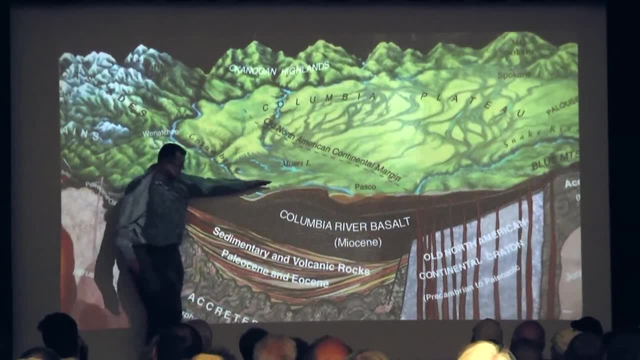 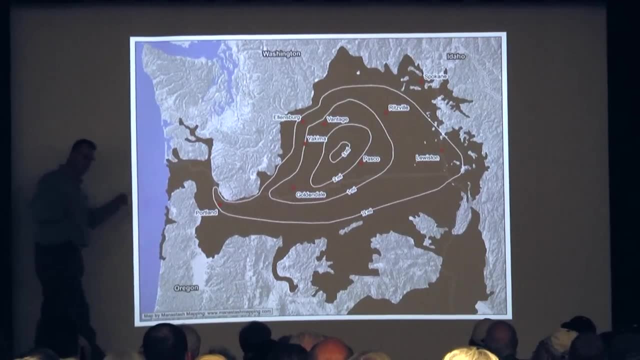 from those I've got a few more and we're done. Let's continue to present in seven days. In one week you can get it as far as. let me just go back. He thinks it takes just seven days to go from here to here all the way to the Dalles and then get that stuff solidified. 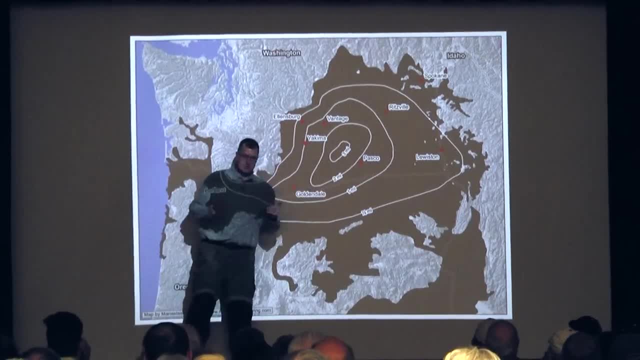 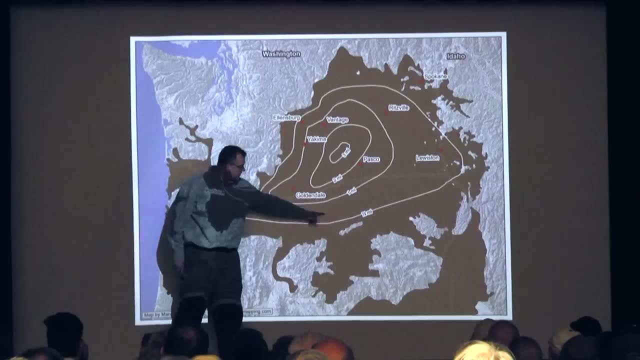 It's tough to approximate this, So there's others that think it takes months. One guy thinks it takes maybe a dozen years or more. Well, we'll maybe never know, but there's maybe new attempts. The Rosa Flow we were just looking at is also famous because it's 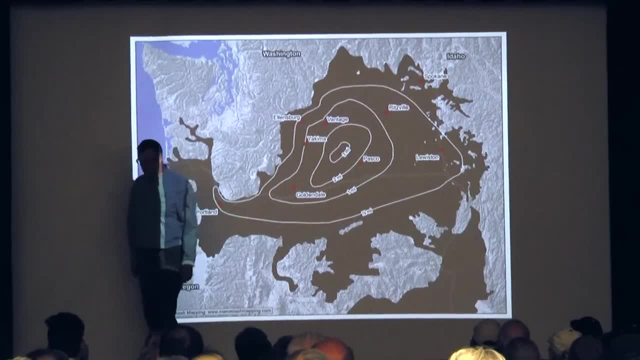 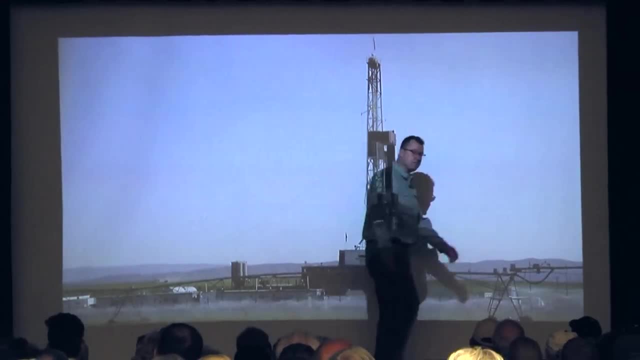 because it makes the beautiful columns of Frenchman Coulee And you've seen rock climbers if you've been to Frenchman Coulee. that's the same flow, That spatter we were just at, that was the vent. Here's the lava being nice and thick and when it cools it cracks and 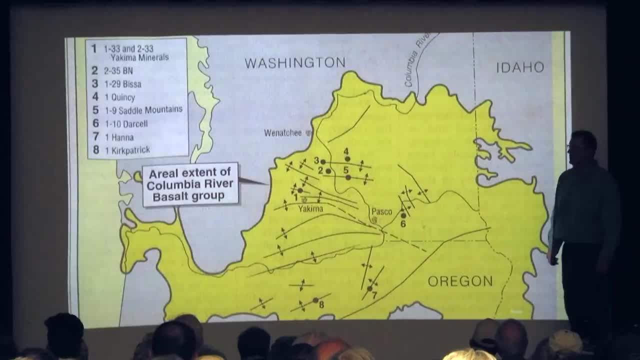 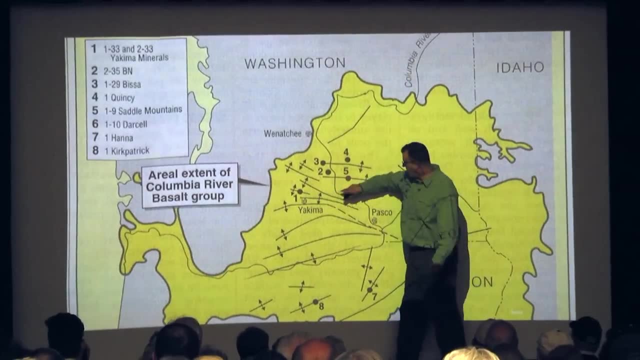 forms these beautiful columns. Not every one of these lava flows forms columns, And it's still a bit of a mystery as to why some of the 300 layers in the German chocolate cake have beautiful columns, others not so well, Plenty of them don't have beautiful columns. 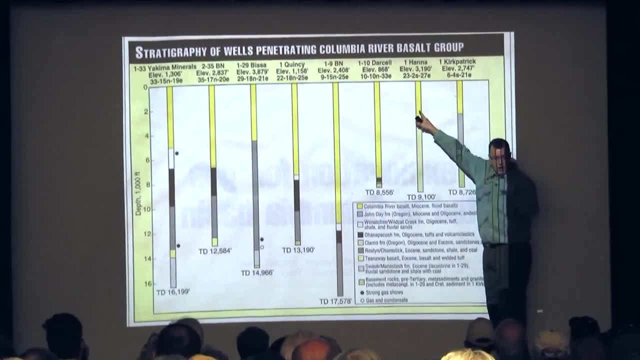 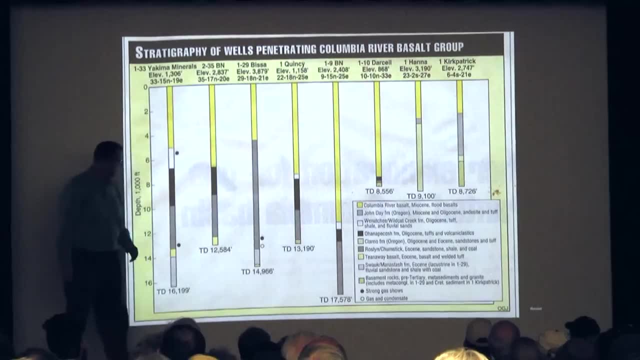 Plenty of others that just don't have columns at all: An upper colonnade, a lower colonnade and an entablature which is kind of a squirrelly cracked zone in the middle. They're all cooling cracks. Priest Rapids Flow actually buried a rhinoceros up in the Grand Coulee called. 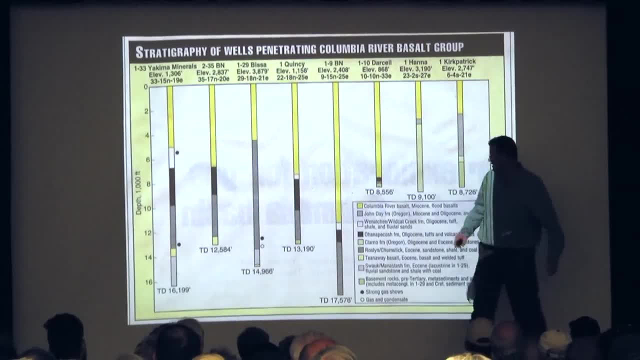 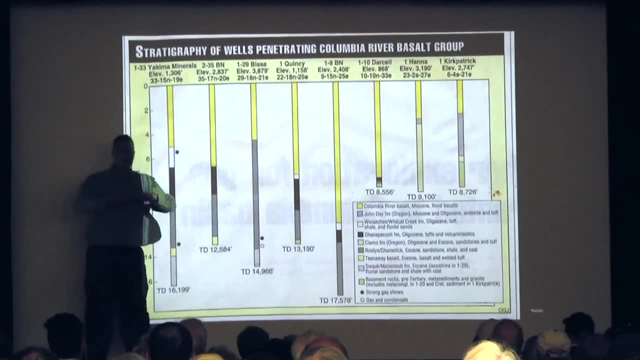 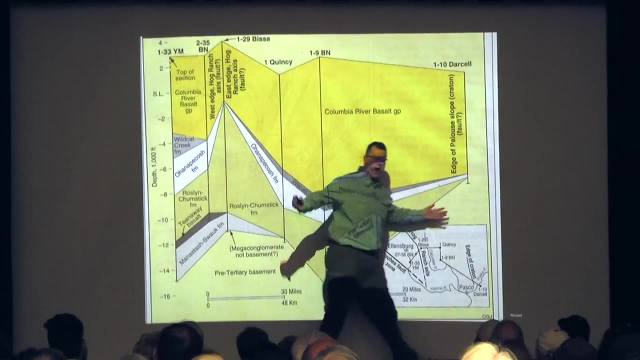 the Blue Lake Rhino. That Priest Rapids Lava Flow made it to Portland and if you've been to the Vista House up above the Columbia, that cliff is this lava flow. So the reason that that cliff is there is there was an old valley that was filled with our basalt lava. 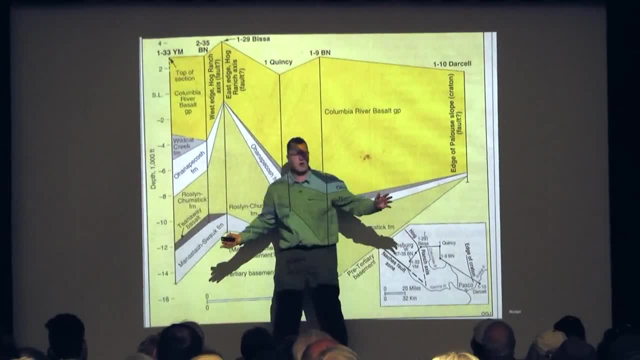 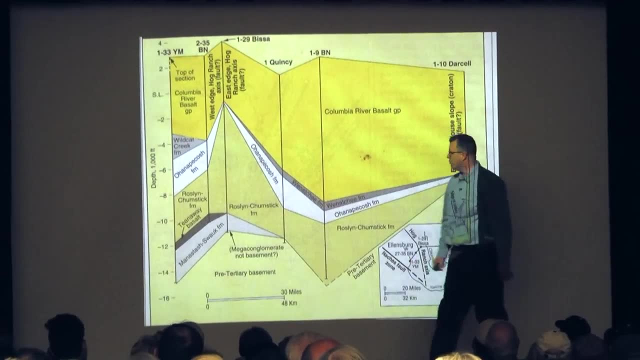 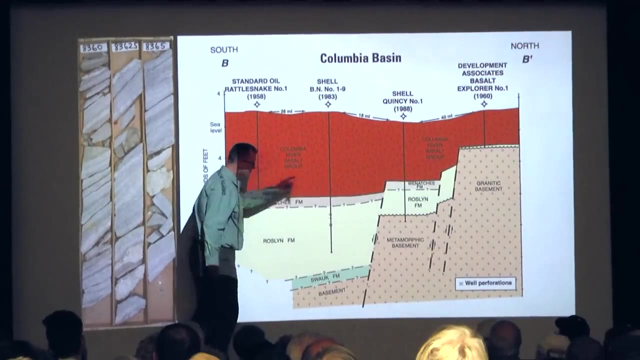 of the Priest Rapids. This is the Umatilla flow coming into Central Washington. This is the Soton. I think I'm starting to lose my concentration here a little bit. God, if I am, are you A couple of these I really like? This is the Pomona lava flow, Some of 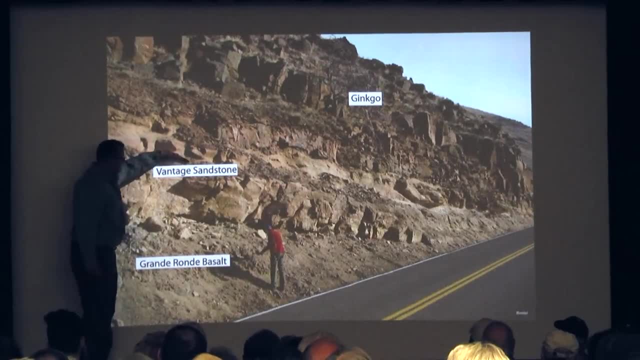 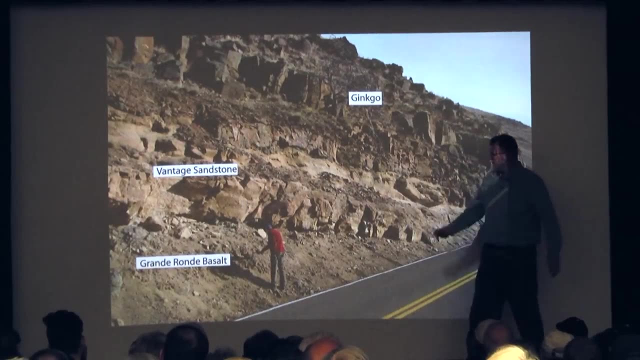 you know the Pomona Lava Flow. A couple of these are really like. this is the Pomona know, the Pomona Tavern maybe, which is just north of Sela. The Pomona cracks opened up over here by Orofino, Idaho. skinny river of orange lava following the old Salmon River. 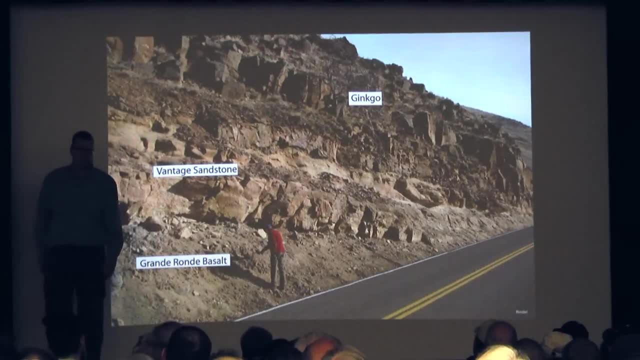 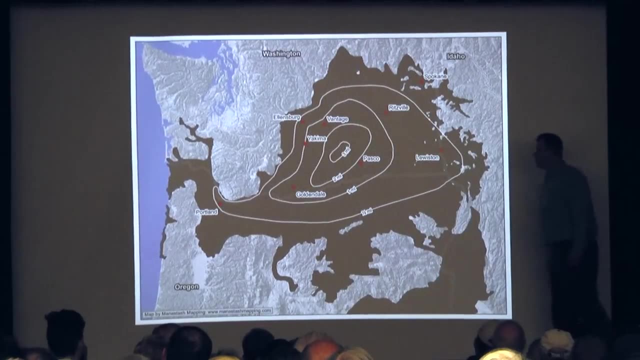 I'm giving away some of the juice from next week. Then the lava spreads into a sheet flow, buries central Washington, finds the Columbia River Valley, funnels back down to it and gets all the way to the Oregon coast. Amazing, That's the Pomona lava flow and this guy. 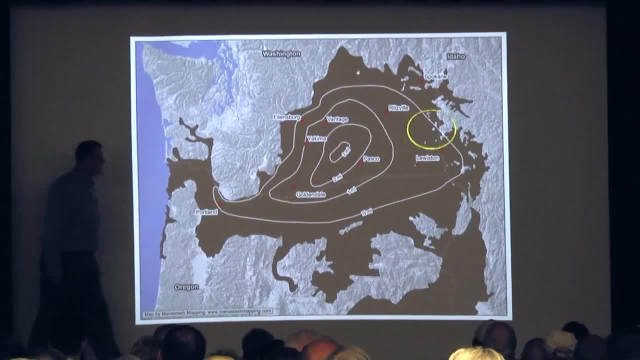 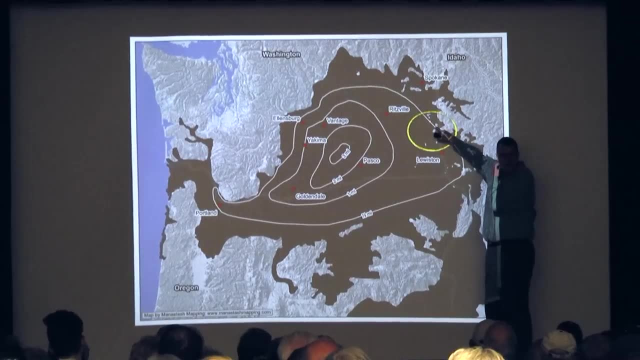 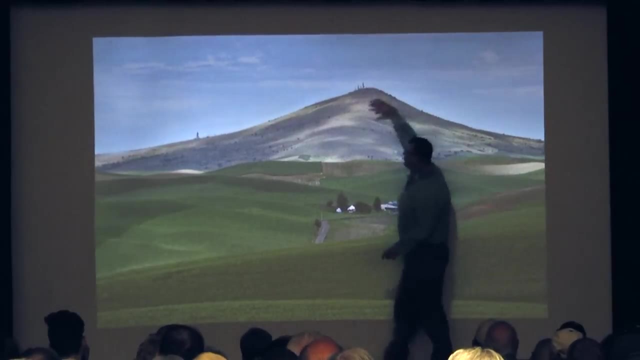 is my favorite. The Elephant Mountain flow A vent down here in northern Oregon. it gets into a river valley and it pools here. Why is the Elephant Mountain my favorite of all the flows? It's photogenic man. The Elephant Mountain is a minor flow. It's not very thick. 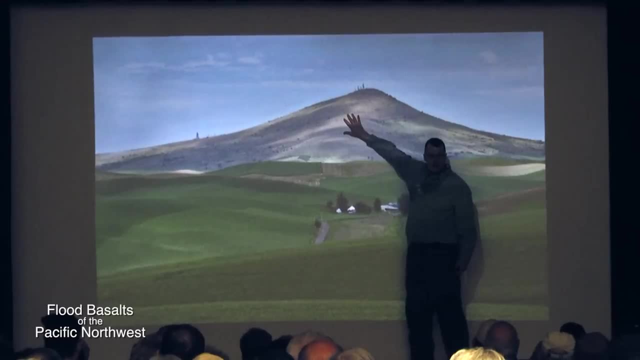 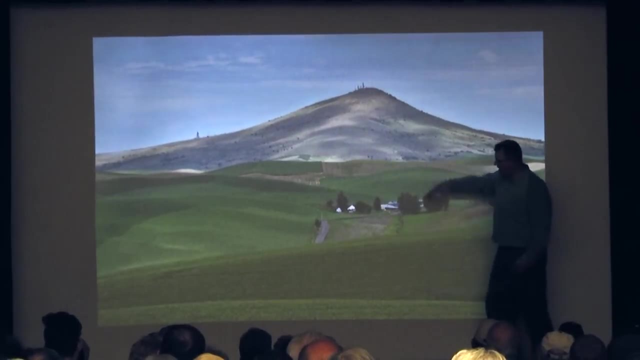 It didn't travel as far as the big boys, but it has the most gorgeous columns and the most beautiful columns. The flow is so thin that you can take people your age. Maybe some of you in the room were out with us. We were out here in April and we were hiking. even though many of us can't, 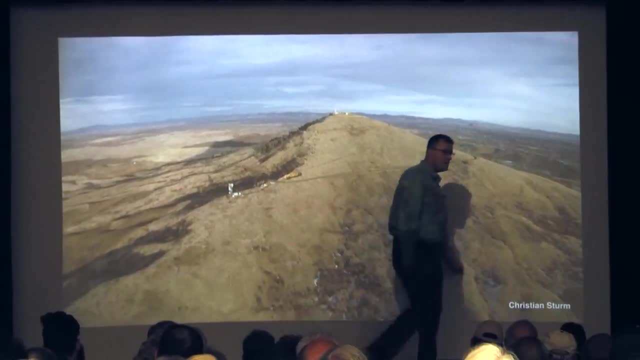 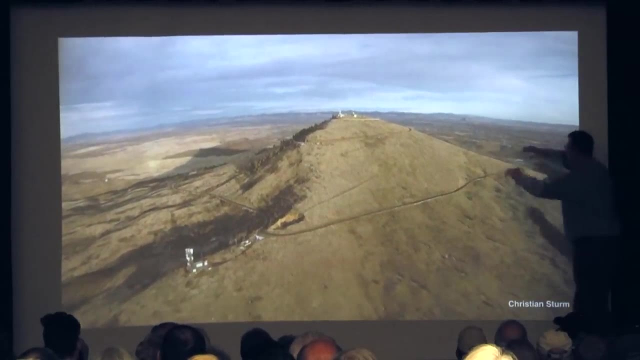 hike very well anymore. We climbed up to the top of the Elephant Mountain flow, going up through these columns and getting up to the top It's an accessible. this is public land as well, near Othello Washington. So here's folks up there. 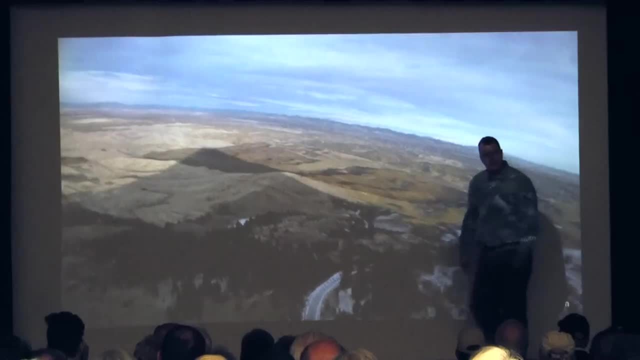 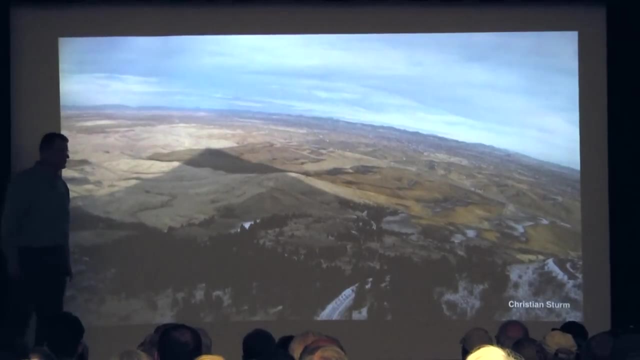 Presiding over these beautiful columns. And if you get up there and look at the tops of these columns, they are so perfectly formed, So beautifully cracked. That's all cooling crack stuff. That's really not the topic of tonight, but I thought I'd include. Oh people. 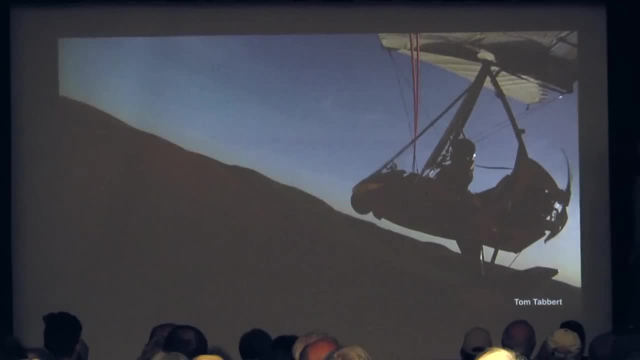 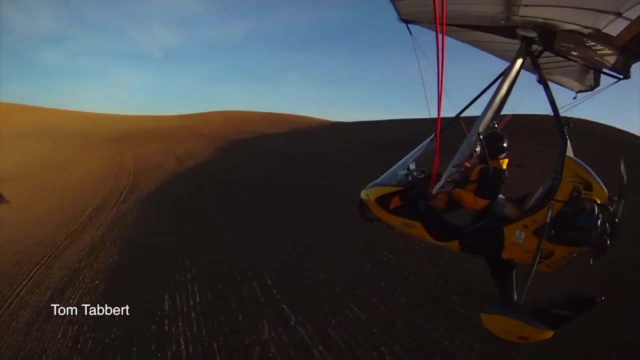 love this. There's lots of talking right now. Look at that, There's a crack. Good Finishing it. Oh, you saw the hammer right. And then this last little guy is the Ice Harbor eruption. I know this isn't six, but close enough. 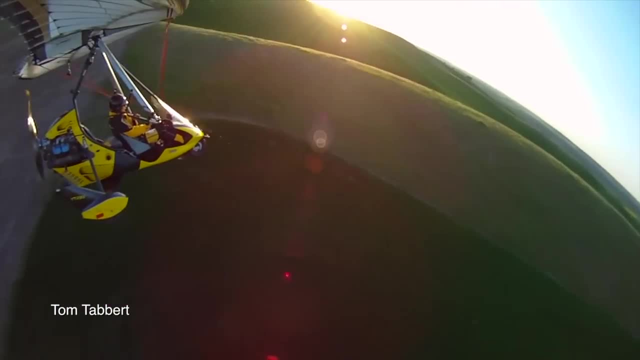 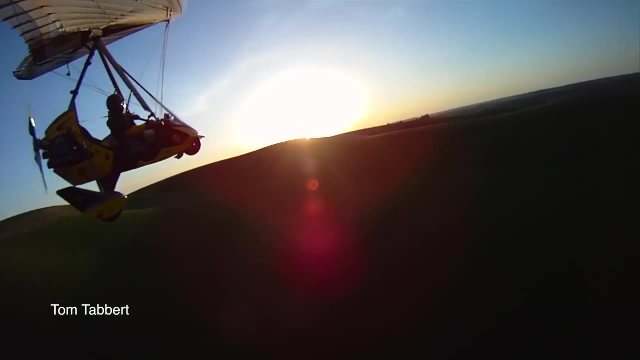 This little guy, the lava got hardly at all. Lewis and Clark came down the Snake and encountered a terrible rapids right here. and that rapids existed Why? Because that feeder dike was sitting right in the Snake River, So even Lewis and Clark were introduced to these Columbia. 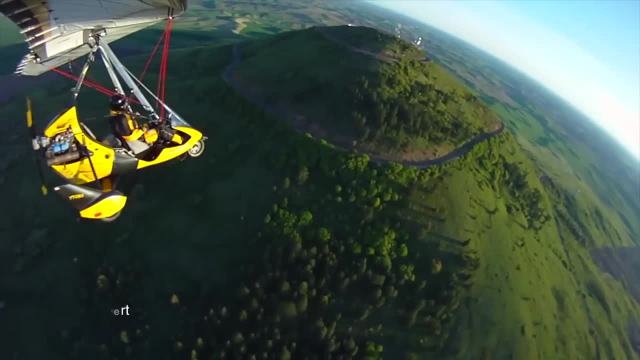 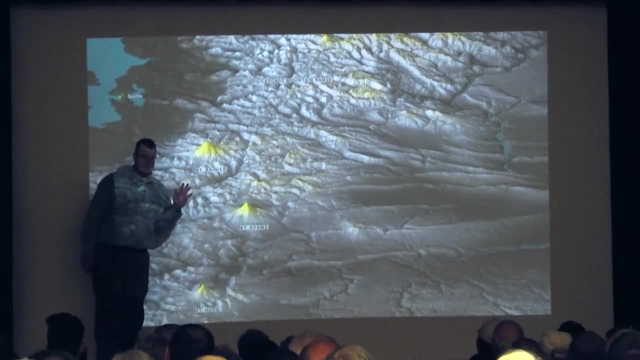 River lavas. I love this diagram because it shows the feeder dikes are not going up to the same horizon And if you think about it, that makes sense right. Here's an older feeder dike. excuse me, here's an older feeder dike feeding an older lava. Now we can see the. 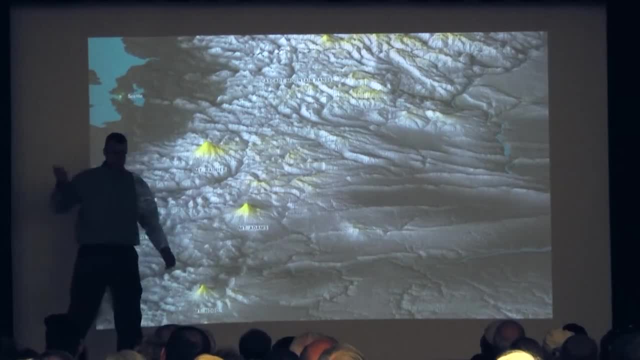 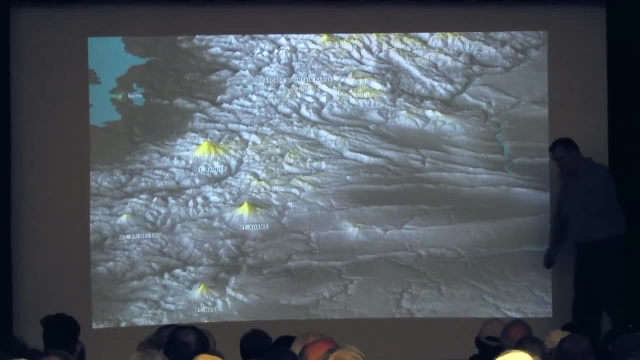 bottom, crack it again, get a younger feeder dike. In other words, you've got to build the layers before you can crack them. So that makes sense if you think about it- At least it did for me, thinking about that recently. Occasionally you find some pillows which 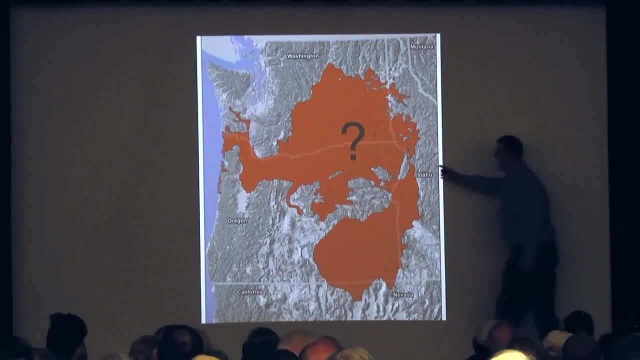 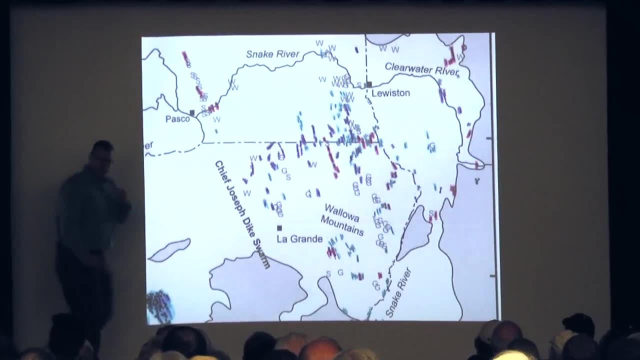 are circular features found only at the bottom of some of these lavas. These pillows tell us that the lava went into a lake of some sort, went into some body of water of some sort, So there's some details preserved there. These are some of the best pillows I've ever. 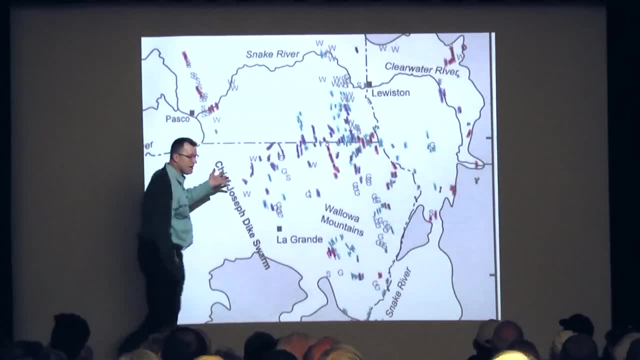 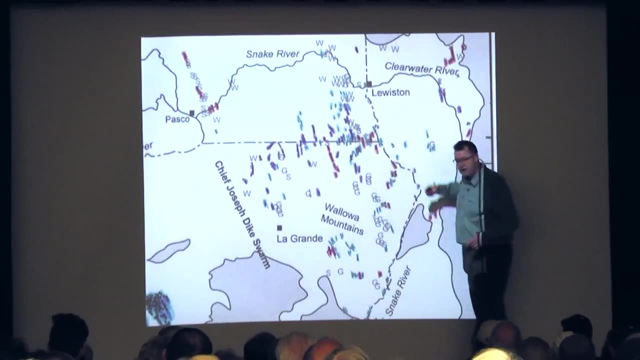 seen. So this is the base of the Priest Rapids flow in downtown Spokane And this is just to the west of downtown. And I think these are amazing because they're kind of three-dimensional. It's not just a highway cut And not every lava flow has the pillows at the base, But 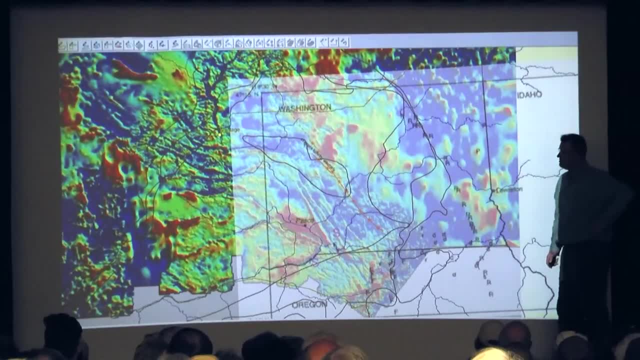 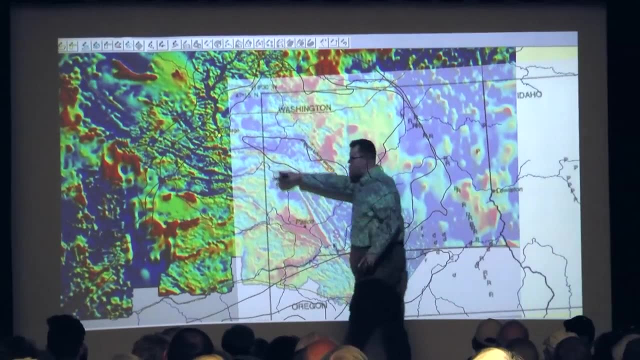 if you find a pillow zone, and then you're extra lucky and you're extra stupid. you get in your vehicle, you drive on the freeway, you cross at Ryegrass, you're heading to Vantage, you pull quickly off to the shoulder. you know that there's some holes, you go crawl. 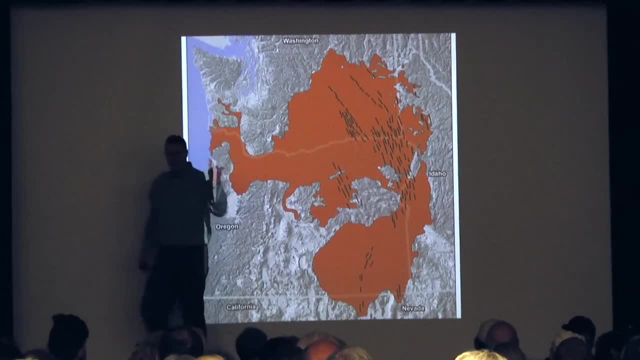 in the holes and you find petrified logs. They're right there. I'm not recommending this State patrol. people will not be happy with me saying that, But you're zooming Every time you drive to Vantage on the freeway. look for those holes down to the south side. 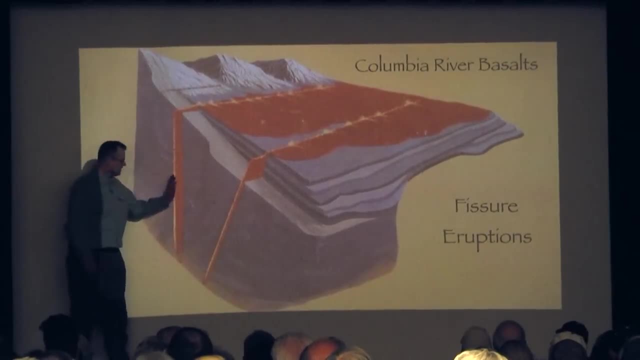 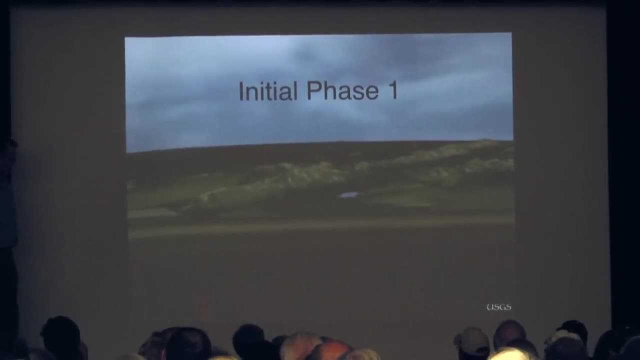 there. so I encourage you. Harrison Sonsen did a good job here by crying out loud. He's a good petroleum expert. They were cool. We have guys that supreme. They're so cool. Finally, we make the tie. Remember we did this early on. We make the tie to the Yellowstone. 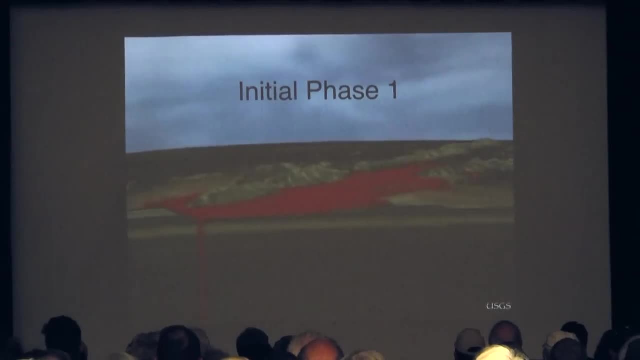 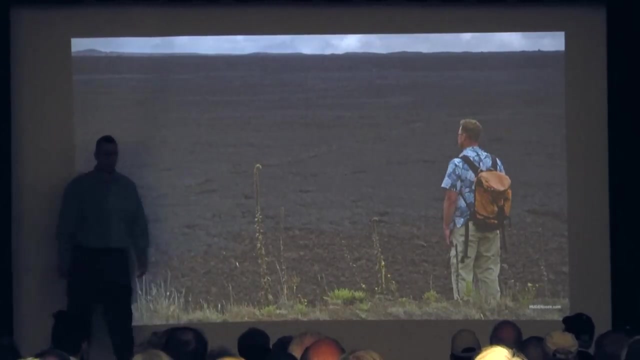 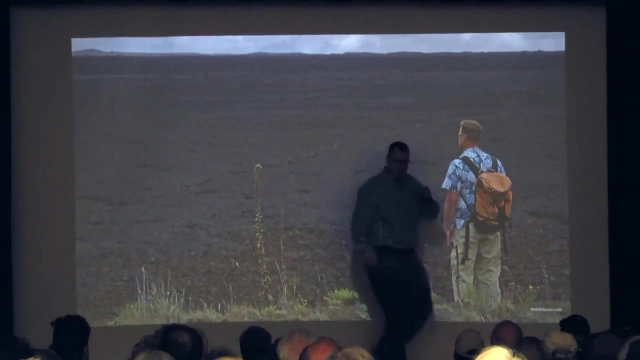 hot spot. Watch this now. We're today in Yellowstone. Let's go back in time until that hot spot is in Northern Nevada 17 million years ago. There are problems, but generally the timing- But generally the timing of that hotspot being here- makes sense for the hotspot story and 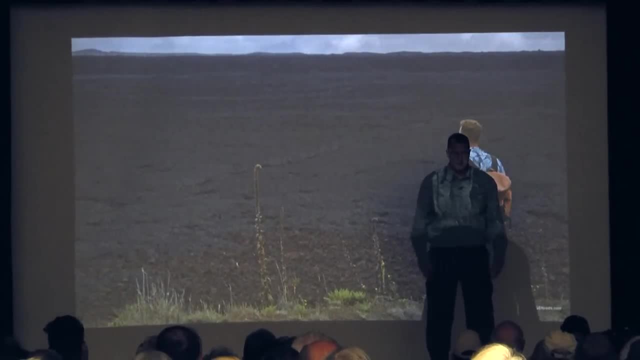 also makes sense for our cracks propagating to the north. And just in case you haven't seen this, you've got a big plume head, a mantle plume head that's upwelling and presumably feeding all of this volcanic activity: 17 to 15 million. 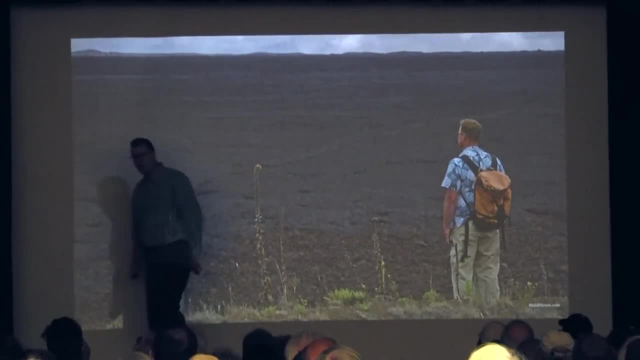 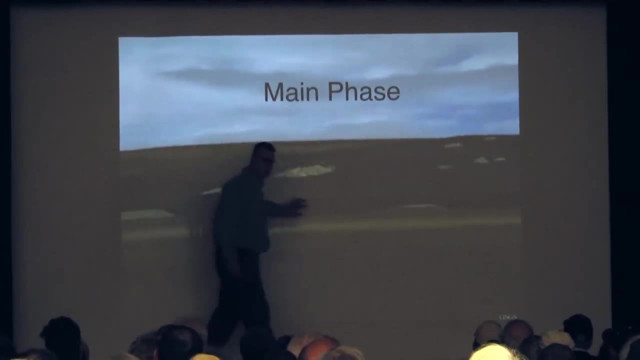 years ago, The Yellowstone story. in case you can't picture, it is this: The stationary Yellowstone hotspot, a drifting North American plate, and you have these incredible explosive calderas, the biggest explosions we've had on planet Earth. all right here. 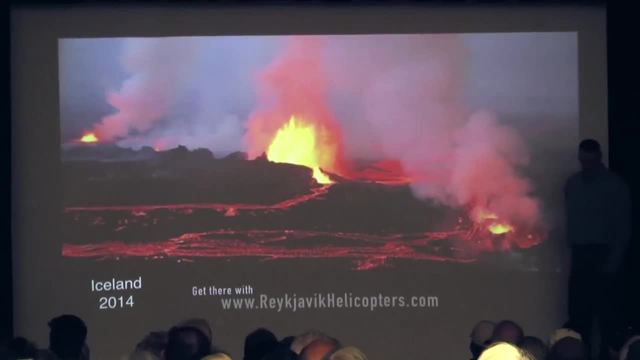 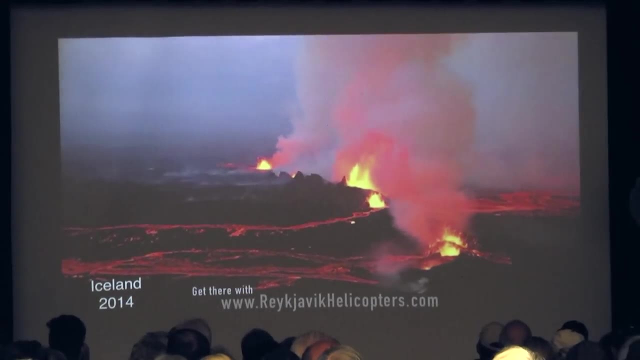 Liz, where you going? All right, My wife taking off. She's had enough. This is North America. It looks like this thing's moving, isn't it? But it's not remember. North America is moving. This is southern Idaho, moving over the stationary hotspot. 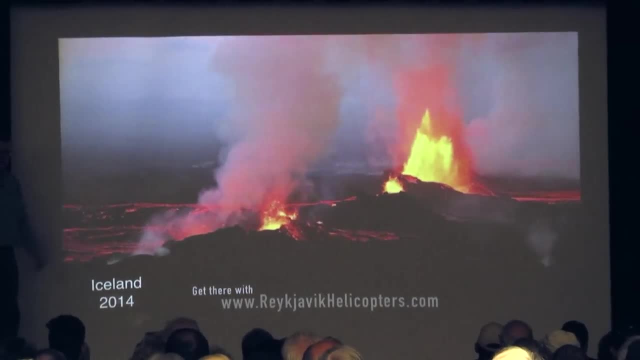 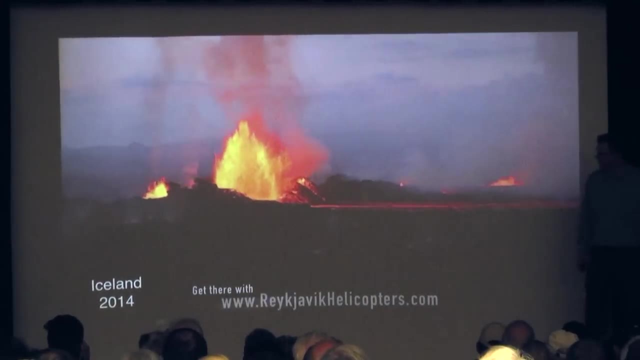 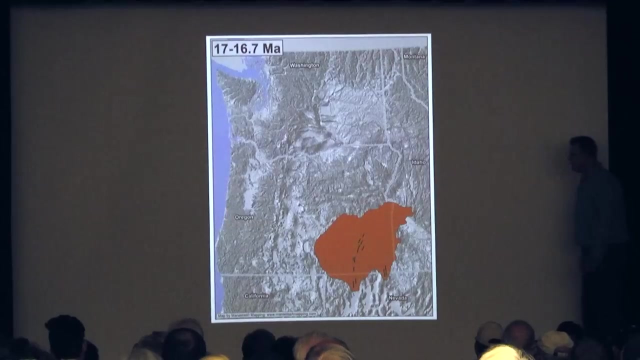 Okay, That's what we visualize, since the hotspot was in the northwest, feeding the basalts. I'd mentioned that these large volcanic regions where we have flood basalts are called large igneous provinces. There's a wonderful book by Richard Ernst. It's pretty technical, but these are just some photos. 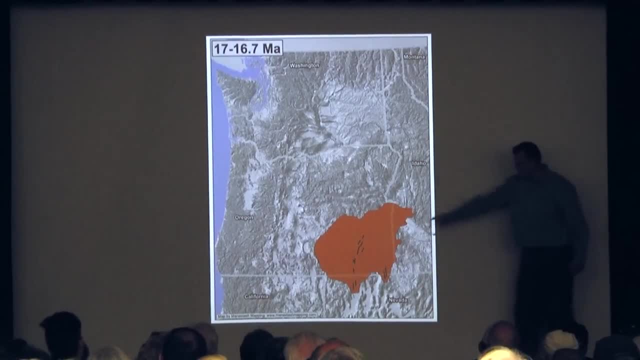 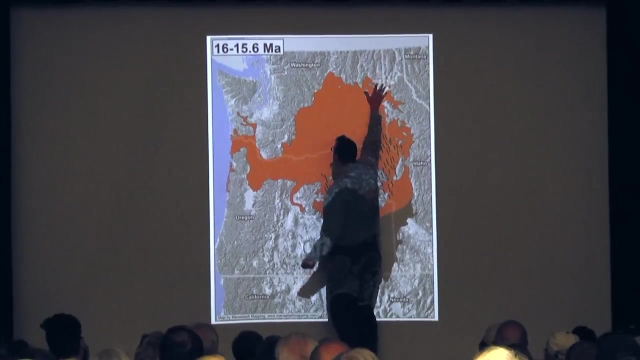 I'm too cheap to buy the book, so I just took some photos out of the book. Each of these black splotches is a basaltic region, A flood basalt region. Here's Siberia, Here's India, Here's the Pangaea flood basalts that are now, of course, separated by the movement. 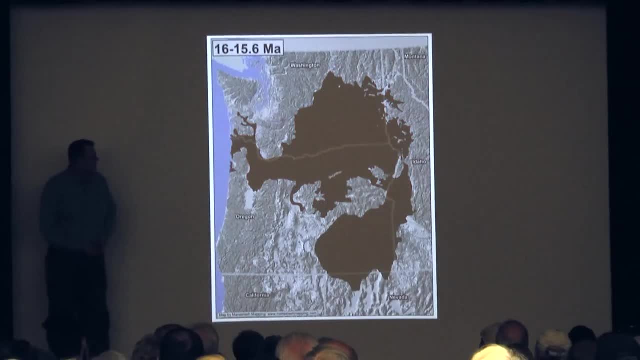 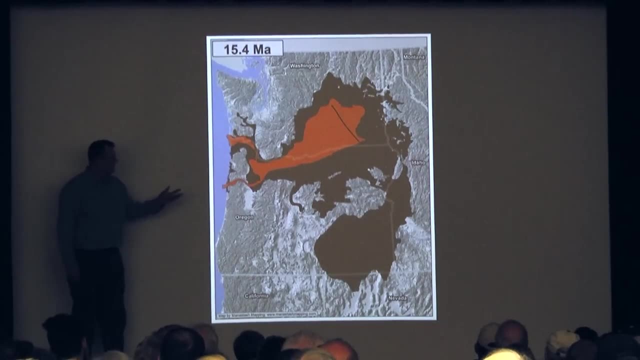 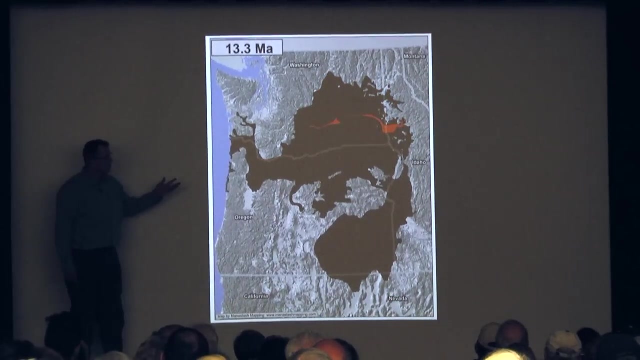 of the continents, but originally they were all together. There are flood basalts in Greenland. There are flood basalts in Siberia. Look at how much Siberia is under basaltic lava. That's the German chocolate cake in Russia. That's Siberia. 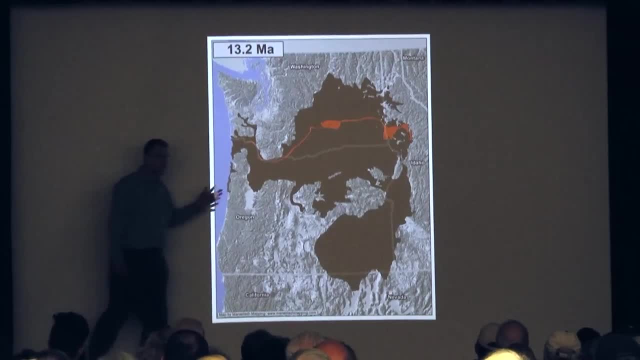 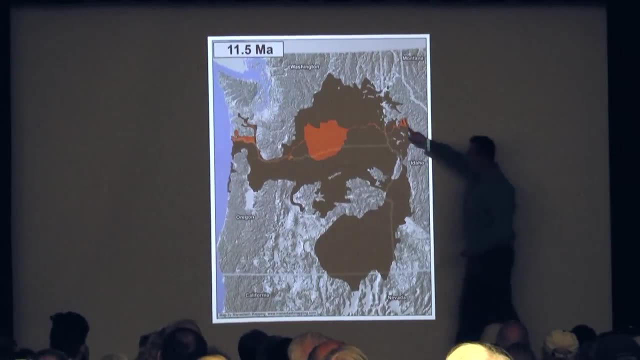 It looks like Yakima Canyon, but it's the flood basalts of Siberia. India- Look at how much of India is buried in flood basalt. many, many more times the volume that we have here. Flood basalts in India.